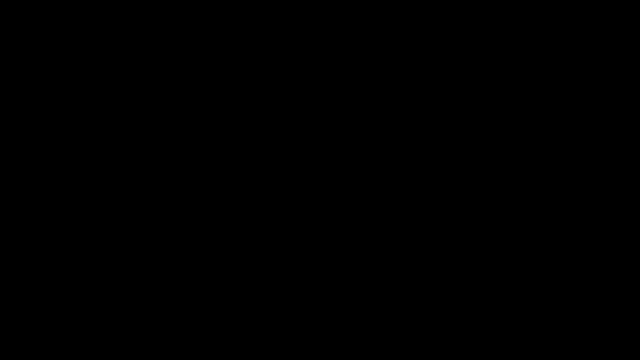 In this video we're going to focus on vectors. What is the difference between a scalar quantity and a vector quantity? What would you say? What's the difference between these two? A scalar quantity has magnitude only, but a vector quantity has magnitude and direction. So, for example, mass is a scalar quantity, but force is a. 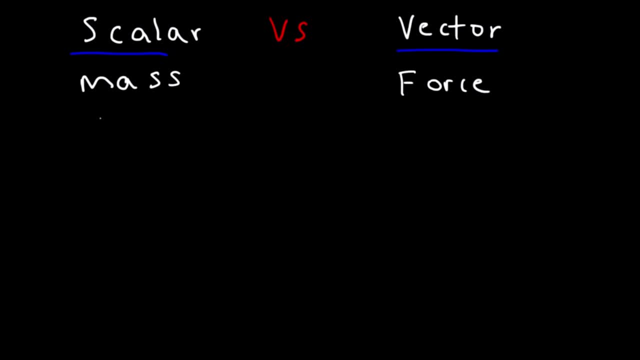 vector quantity. For example, let's say you have a mass of 30 kilograms. You can't say you have 30 kilograms directed east or 70 kilograms directed north. That doesn't make sense. So the 30 kilograms is the magnitude, but there's no direction. 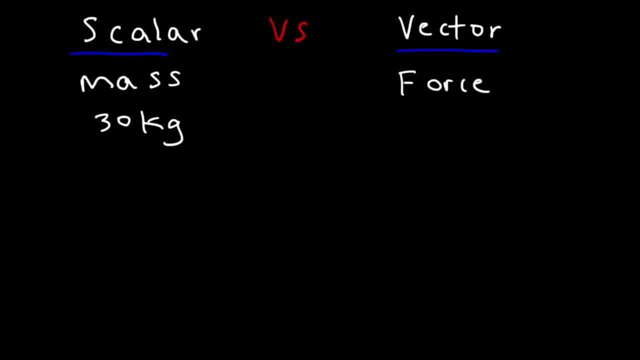 that's relevant to it. So that's why mass is a scalar quantity. You can't have direction with mass. However, force is a vector quantity. I can push an object with a force of 200 newtons directed east, or I can lift up an object with a force of 300 newtons. 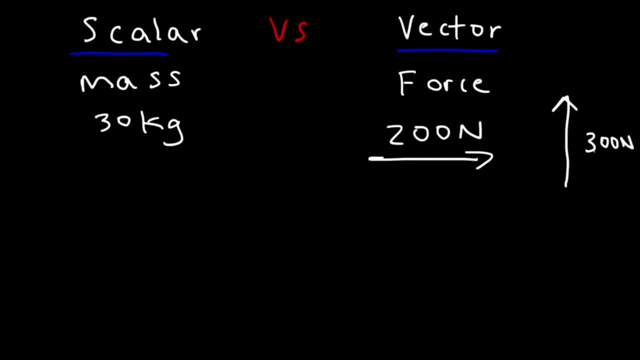 directed up. So therefore, force has magnitude and direction. So if I direct a force of 80 newtons at an angle of 30 degrees above the x-axis, the magnitude is the 80 newtons, The angle the 30 degrees. that's the direction. 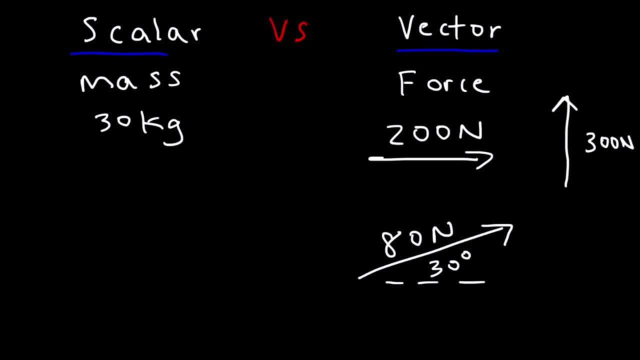 So other examples of vector quantities are velocity, velocity of speed with direction and acceleration, which is how fast velocity is changing. Speed is scalar and temperature is also a scalar quantity. Let's say, if we have an initial point, point A, which is at 1,, 2, and a terminal, 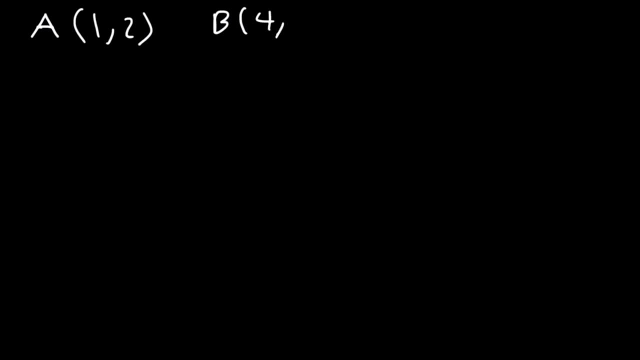 point, point B, which is going to be at 4, 6.. And let's say, vector V is the directed line segment from A to B. How can you express vector V in terms of its components i and j? And also, how can you find the magnitude of vector V? 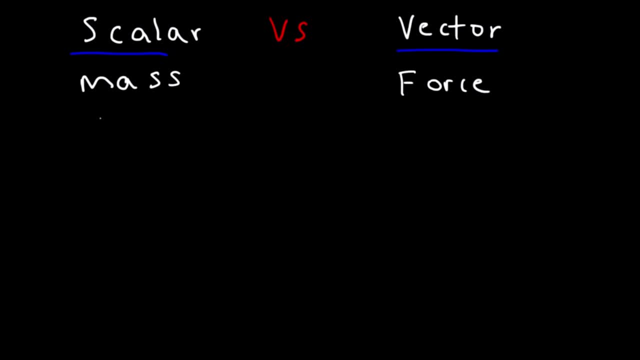 vector quantity. For example, let's say you have a mass of 30 kilograms. You can't say you have 30 kilograms directed east or 70 kilograms directed north. That doesn't make sense. So the 30 kilograms is the magnitude, but there's no direction. 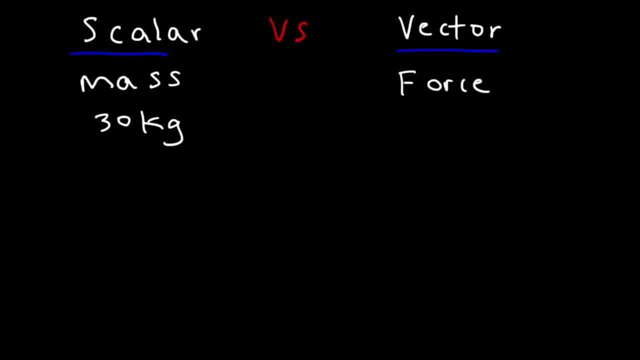 that's relevant to it. So that's why mass is a scalar quantity. You can't have direction with mass. However, force is a vector quantity. I can push an object with a force of 200 newtons directed east, or I can lift up an object with a force of 300 newtons. 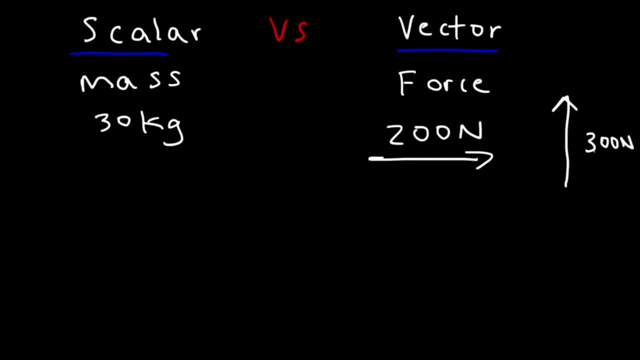 directed up. So therefore, force has magnitude and direction. So if I direct a force of 80 newtons at an angle of 30 degrees above the x-axis, the magnitude is the 80 newtons, The angle the 30 degrees. that's the direction. 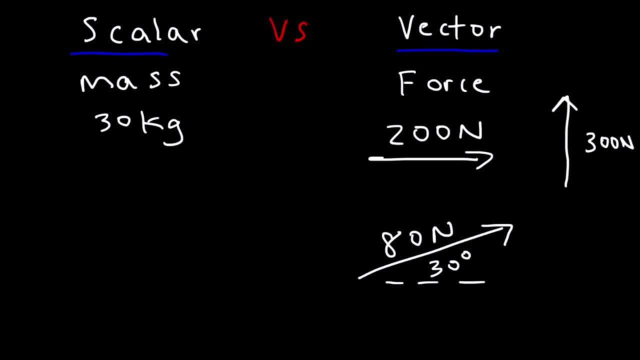 So other examples of vector quantities are velocity, velocity of speed with direction and acceleration, which is how fast velocity is changing. Speed is scalar and temperature is also a scalar quantity. Let's say, if we have an initial point, point A, which is at 1,, 2, and a terminal, 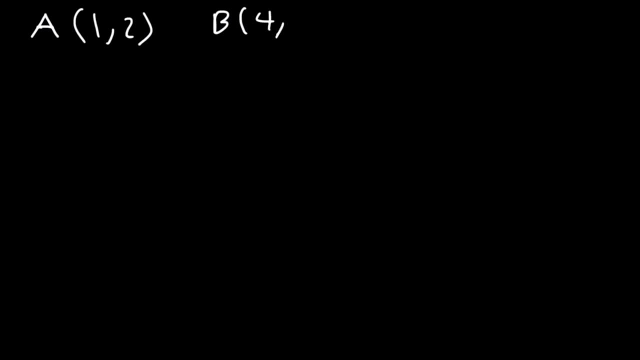 point, point B, which is going to be at 4, 6.. And let's say, vector V is the directed line segment from A to B. How can you express vector V in terms of its components i and j? And also, how can you find the magnitude of vector V? 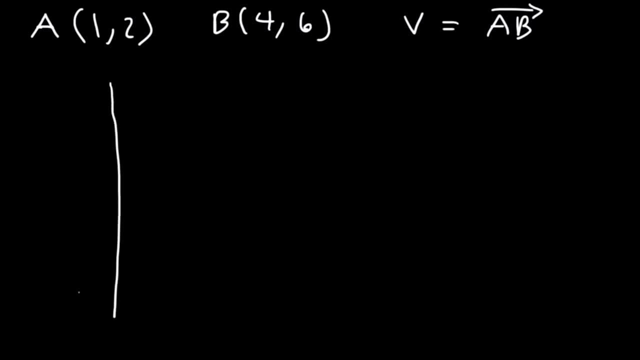 Well, first let's draw a graph. The majority of the graph will be in the first quadrant, So A is at 1, 2.. So this is point A, And B is at 4, 6, which is about that point. 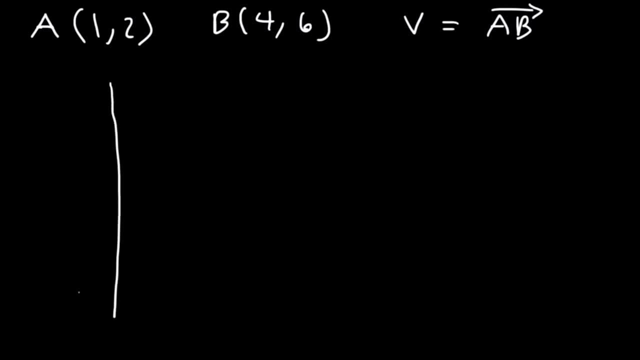 Well, first let's draw a graph. The majority of the graph will be in the first quadrant, So A is at 1, 2.. So this is point A, And B is at 4, 6, which is about that point. 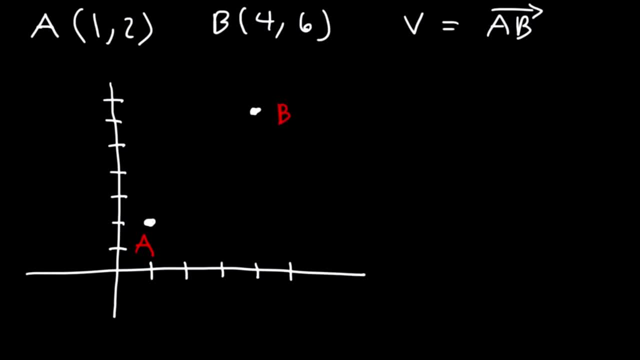 The vector V extends from the initial point A to the terminal point B. The left of that line is the magnitude of vector V. Now if we take the difference in the x-values, that is, if we subtract 4 and 1, we're going to get 3, which means to go. 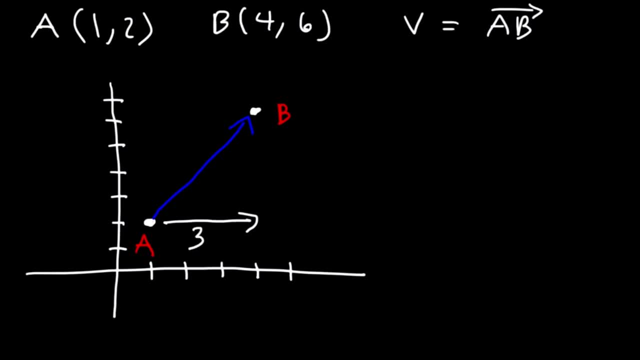 from A to B, we have to travel three units to the right And we need to go up four units. Those are the components of vector V, So vector V can be expressed as 3i plus 4j. i is associated with the x-component of. 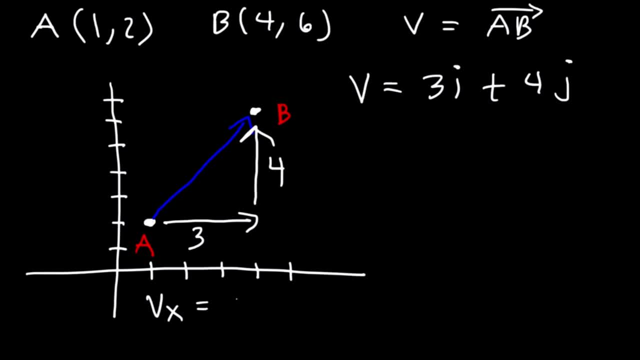 vector V. So you could say Vx is 3.. The y-component of vector V is 4, which is associated with the letter j. Now to find the magnitude of vector V, you can use this equation: V is the square root. 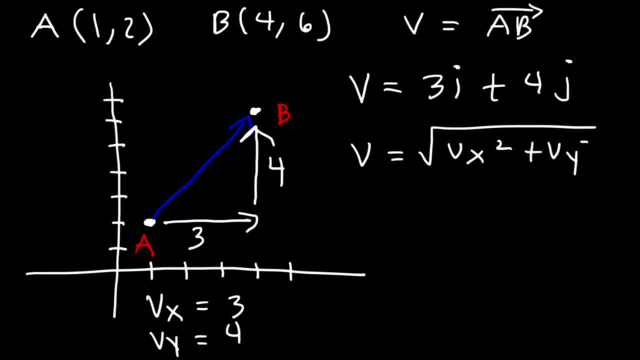 of Vx squared plus Vy squared- This comes from the Pythagorean Theorem- C is equal to the square root of A squared plus B squared. So vector V is going to be the square root of 3 squared plus 4 squared, And that's going to give us the length of the hypotenuse. 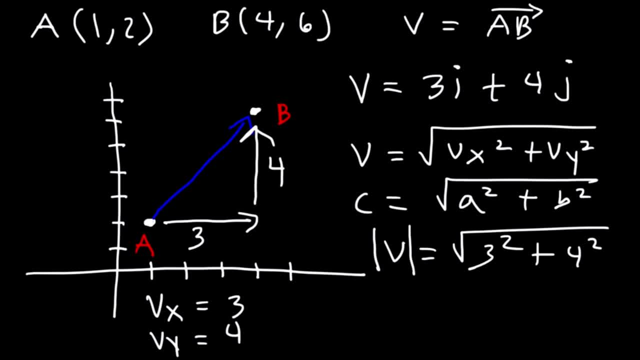 By the way, when you see this inside an absolute value, it represents the magnitude of V. by the way, 3 squared is 9.. 4 squared is 16.. 9 plus 16 is 25.. And the square root of 25 is 5.. 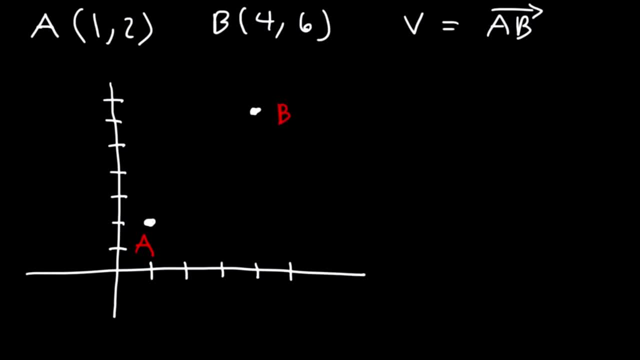 The vector V extends from the initial point A to the terminal point B. The left of that line is the magnitude of vector V. Now if we take the difference in the x-values, that is, if we subtract 4 and 1, we're going to get 3, which means to go. 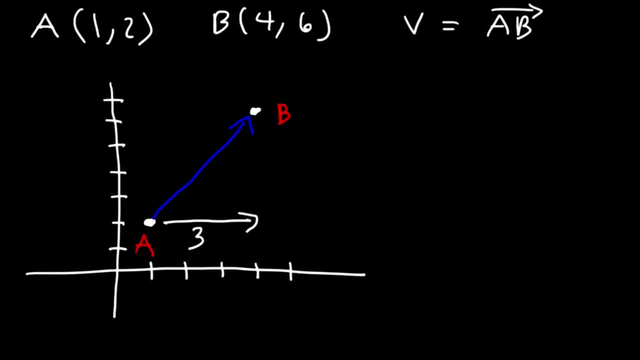 from A to B, we have to travel three units to the right And we need to go up four units. Those are the components of vector V, So vector V can be expressed as 3i plus 4j. i is associated with the x-component of vector V, So you can. 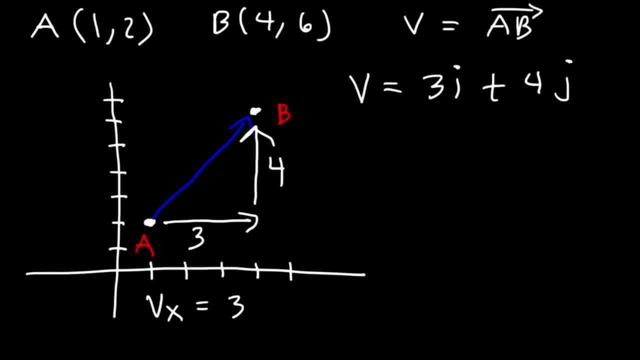 say Vx is 3.. The y-component of vector V is 4, which is associated with the letter V. Now to find the magnitude of vector V, you can use this equation: V is the square root of Vx squared plus Vy squared. This comes from the Pythagorean Theorem. C is 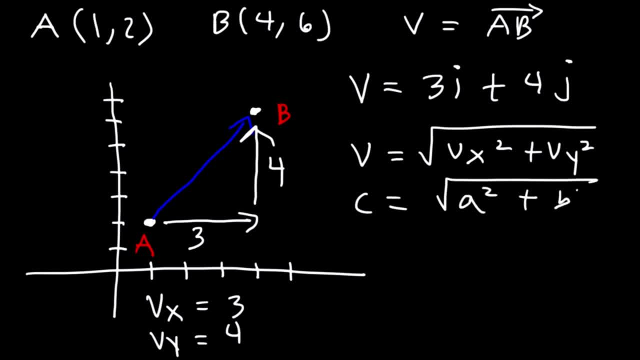 equal to the square root of A squared plus B squared. So vector V is going to be the square root of 3 squared plus 4 squared, And that's going to give us the length of the hypotenuse. By the way, when you see this inside an absolute value, it represents the magnitude of V. by the way, 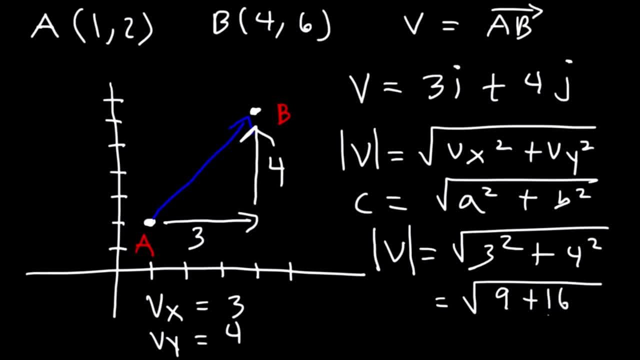 3 squared is 9.. 4 squared is 16.. 9 plus 16 is 25.. And the square root of 25 is 5.. So the magnitude of vector V is 5.. So this line is basically 5 units long. 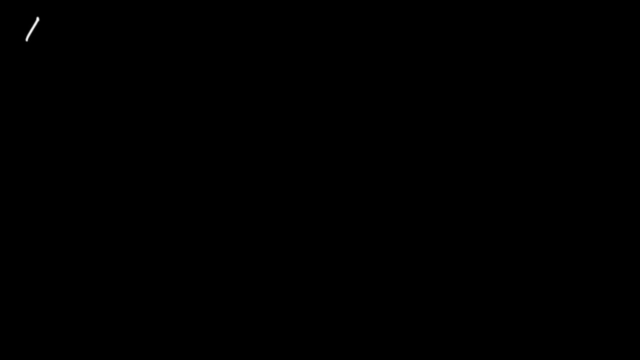 Let's try another problem. So let's say that point A is located at negative 4, negative 5. And point B is located at 1 comma 7.. Go ahead and express vector V in terms of its components i and j and find the magnitude. 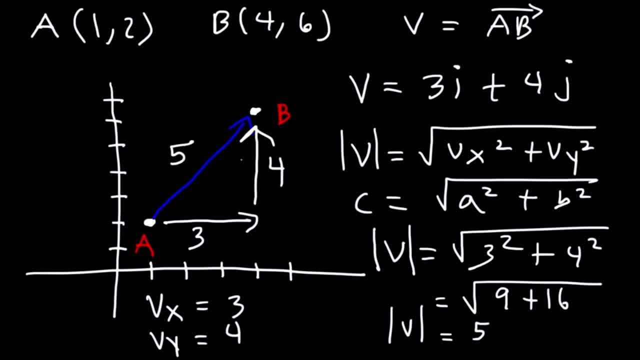 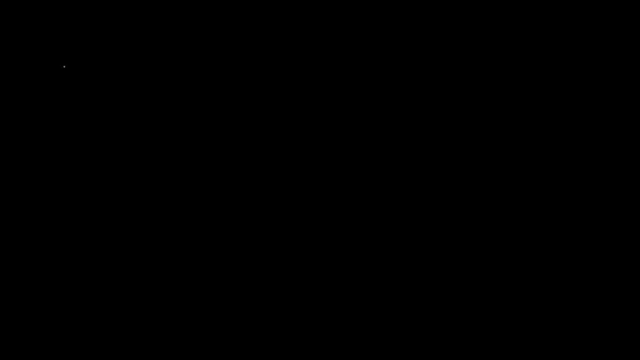 So the magnitude of vector V is 5.. So this line is basically 5 units long. Let's try another problem. So let's say that point A is located at negative 4, negative 5. And point B is located at 1 comma 7. Go. 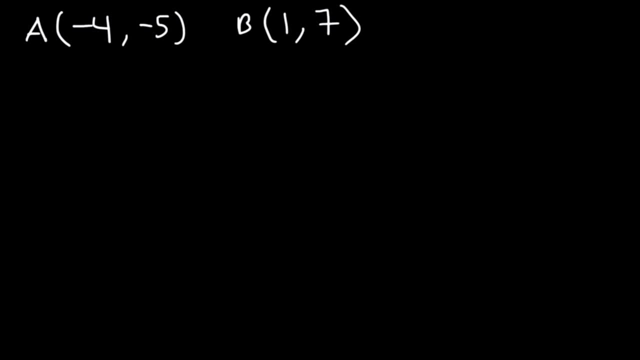 ahead and express vector V in terms of its components i and j and find the magnitude. So let's call this x1 and x2.. And this is y1 and y2.. If you don't want to graph it, you can use this equation. 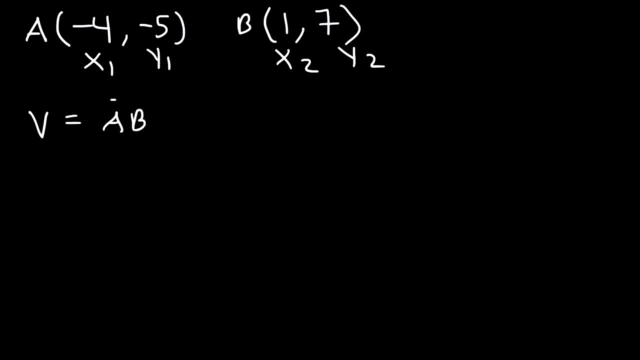 So vector V, which is the directed line segment from A to B- and let's say A, once again, is the initial point and B is the terminal point- It's going to be the difference in the x values and that's going to give us the i component or the x component, and then we have the difference. 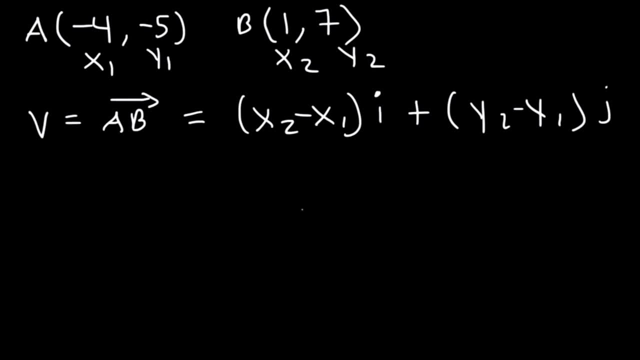 in the y values, which gives us 1, and at a, And so vector B is the directed line, component values. that's going to give us the y component which is associated with J. so x2 minus x1, that's going to be 1 minus negative 4 and y2 minus y1, so that's 7. 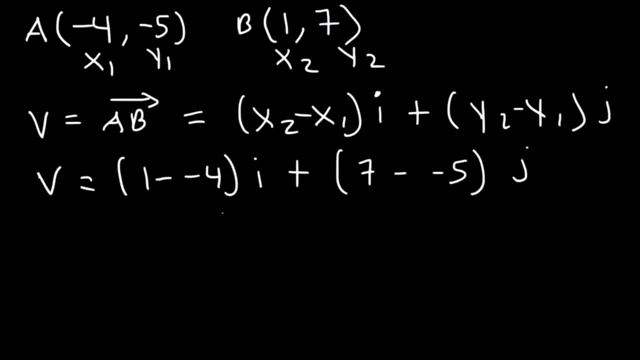 minus negative 5. so 1 minus negative 4 is the same as 1 plus 4, that's 5. 7 minus negative 5, that's 12. so we have 5i plus 12 J. so that's the vector V expressed in. 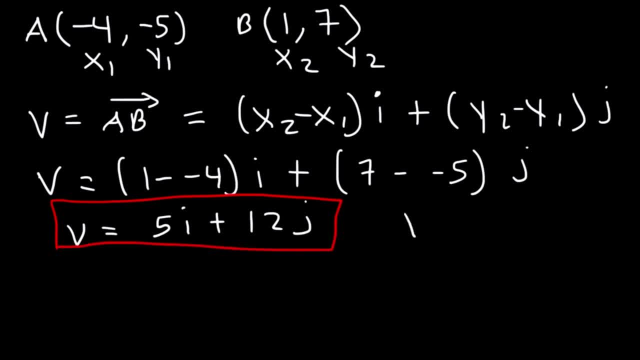 its components. now we can also represent vector V this way as well. you can say: it's 5 comma 12. so that's another way you can express it. now let's find the magnitude of vector V. so it's going to be the square root of 5 squared plus 12. 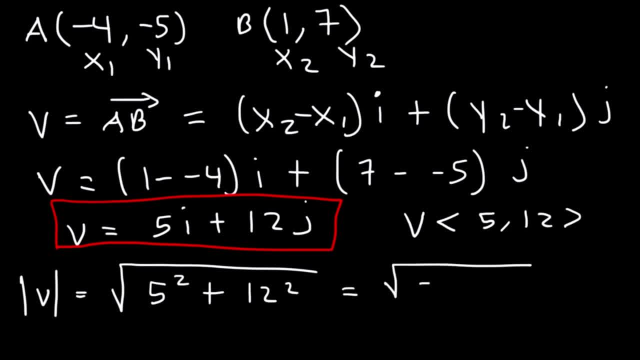 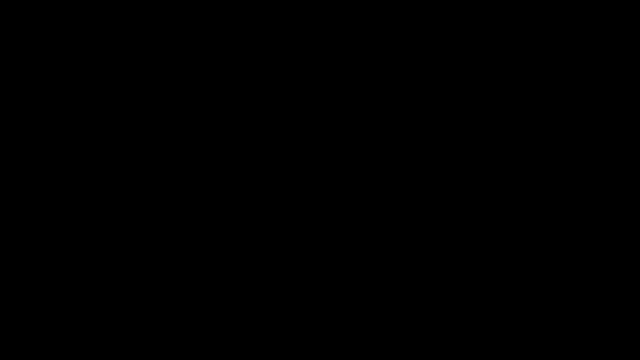 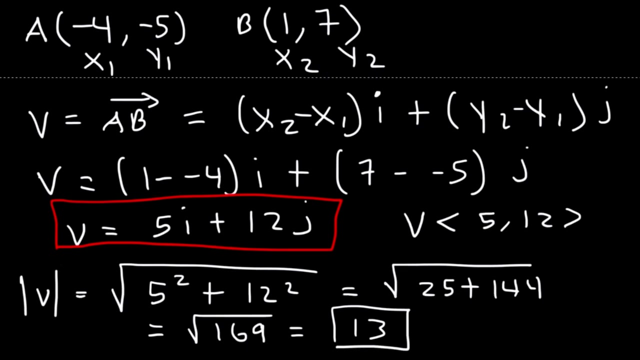 squared 5 squared is 25, 12 squared is 144, and 25 plus 144 is 169. so this is going to be 13. so that's the magnitude of vector V. now you can also get the same answer by graphing it as well. 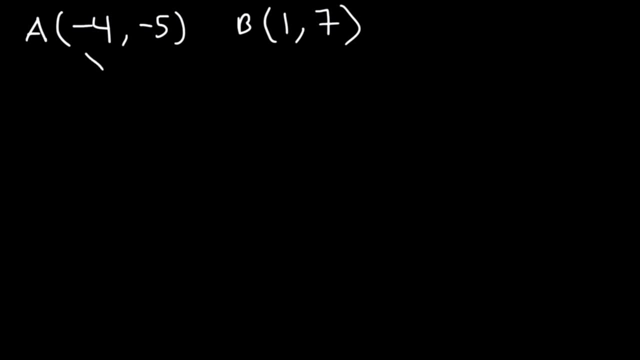 So let's call this x1 and x2.. And this is y1 and y2.. If you don't want to graph it, you can use this equation. So vector V, which is the directed line segment from A to B, and let's say A once again. 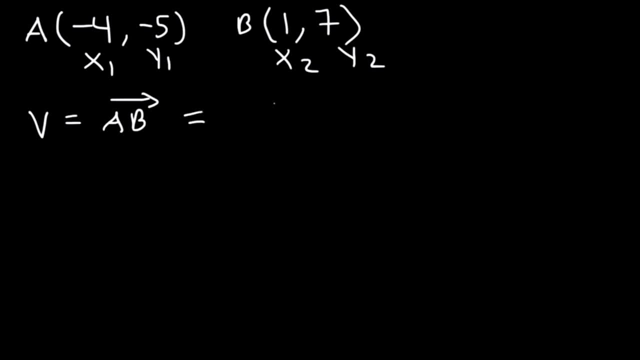 is the initial point and B is the terminal point. it's going to be the difference in the X values, and that's going to give us the i component or the X component. And then we have the difference in the y values that's going to give us the y component. 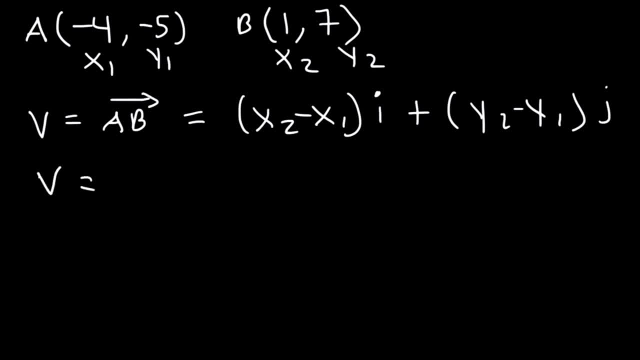 which is associated with J. so X 2 minus X 1, that's going to be 1 minus negative 4, and y 2 minus y 1, so that's 7 minus negative 5. so 1 minus negative 4 is the same as 1 plus 4, that's 5. 7 minus negative 5, that's 12, so we have 5, I plus. 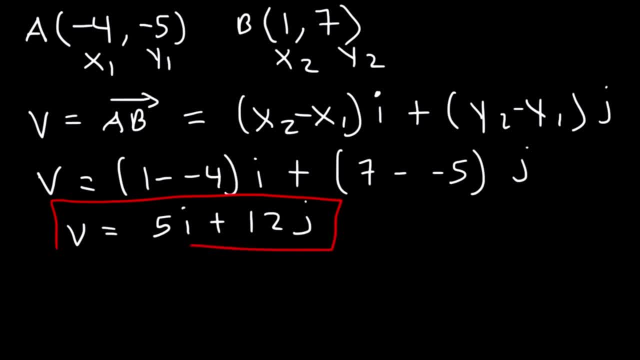 12, J. so that's the vector V expressed in its components. now we can also represent vector V this way as well. you can say it's 5 comma 12, so that's another way you can express it. now let's find the magnitude of vector V. so it's going to 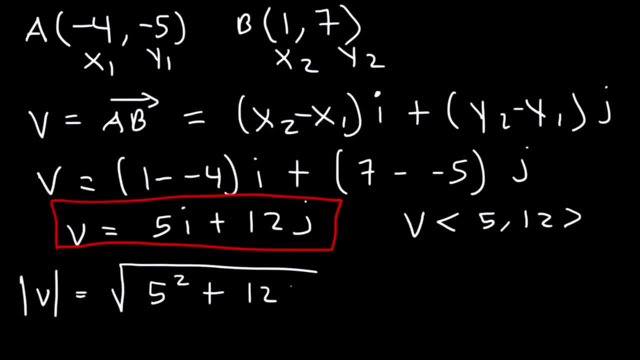 be the square root of 5 squared plus 12 squared. 5 squared is 25, 12 squared is 144, and 25 plus 144 is 169. so this is going to be 13. so that's the magnitude of vector V. now you can also get the same answer by graphing it as well. 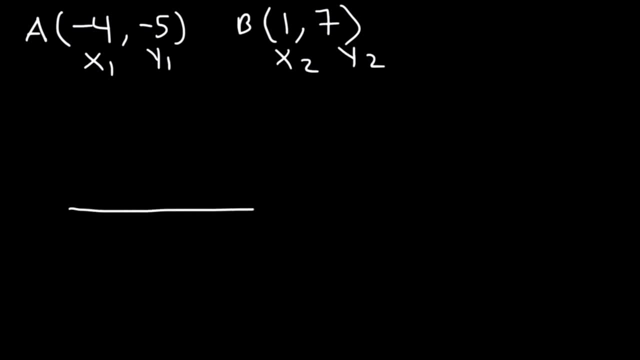 so a is that negative 4, negative 5, and B is that one seven. so here's B, so here's negative 4, and this is positive one. so we have to travel five units to the right, and then, from a y value of negative 5 to 7, we have to. 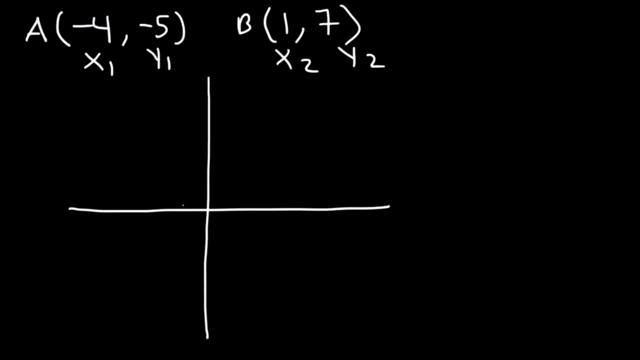 you can also get the other side of thelaşed come. this is going to be the gradient one. if you have the third, the 140th. so let's say that we get this 총 form okay. so if you have three tops, that exactly the same. so you can always. 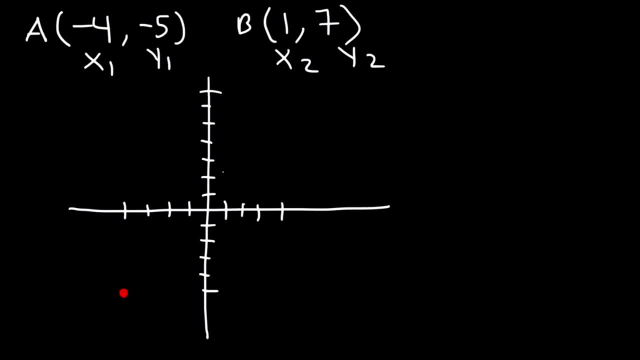 put your two or make them equal Babel. So let's just say the material that we need, because it has that number and we can write it by putting it here too, see, and this is positive 1. So we have to travel 5 units to the right, And then from a y value of 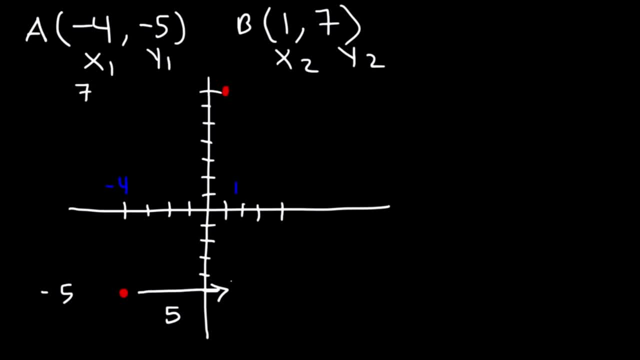 negative 5 to 7, we have to travel 12 units up, So that's why the vector is 5i plus 12j, And then the magnitude or the distance between the initial point A and B is 13 units apart. 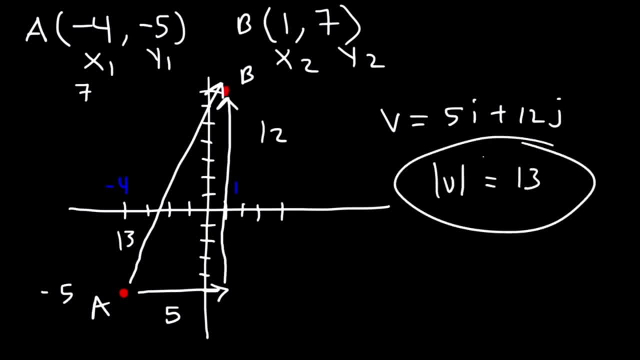 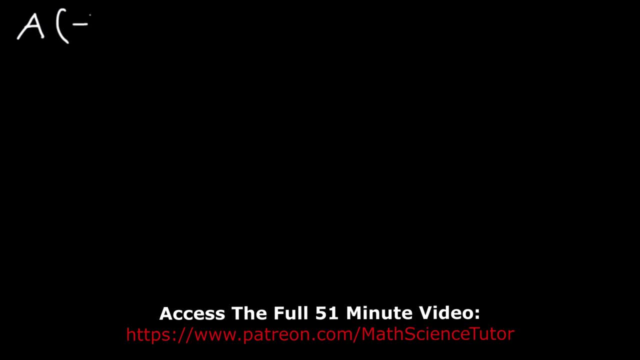 So the magnitude of vector V is 13.. Now here's a question for you. Let's say, if we have the initial point A, which is at negative 1,, negative 3. And you're given the vector V, which is the directed line segment from A to B, 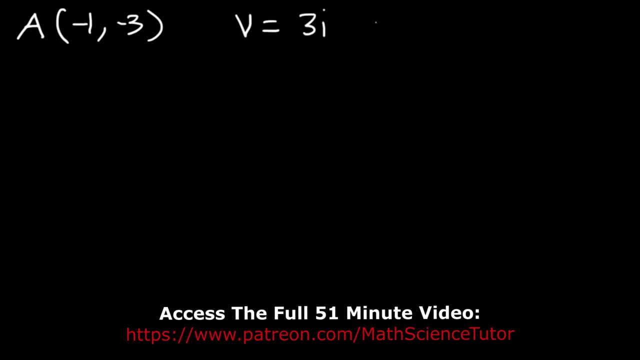 And let's say it's 3i minus 2j, What is point B? if A is the initial point and B is the terminal point? How can you use vector V to find the answer? Well, you can get the answer graphically. 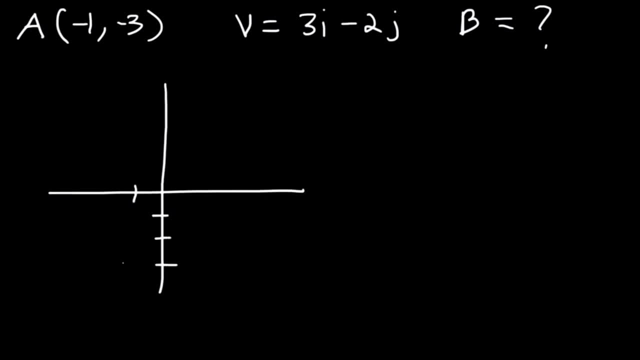 First let's plot vector A, So it's at negative 1,, negative 3.. And then we can use vector V to find the answer. So we can use vector V to find the answer, And then we can use vector V to find the answer. 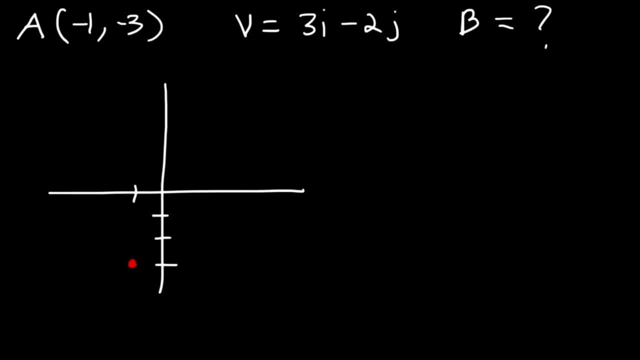 And then we can use vector V to find point B. So notice that we have positive 3i. That means from A we need to travel 3 units to the right, So we're at an x value of negative 1. If we add 3 to it, 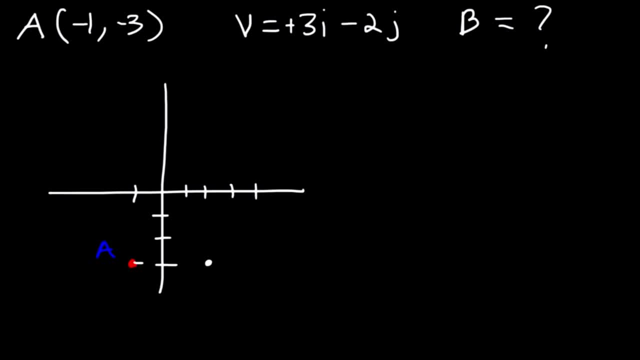 it's going to take us to this point here. So we travel 3 units to the right. Now notice that there's a negative 2 in front of j, which means we need to go down 2 units. So therefore, this is point B. 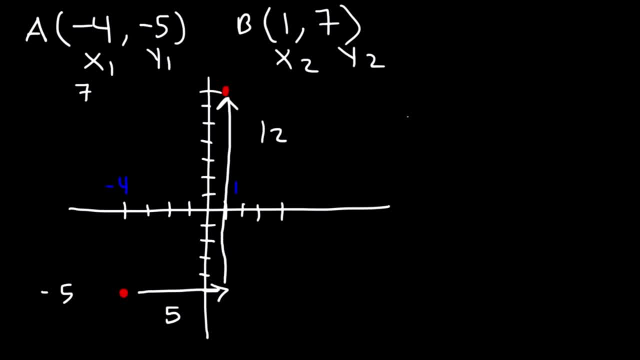 travel 12 units up, so that's why the vector is 5i plus 12 J. and then the magnitude or the distance between the initial point a and b is 13 units apart, so the magnitude of vector V is 13. now here's a. 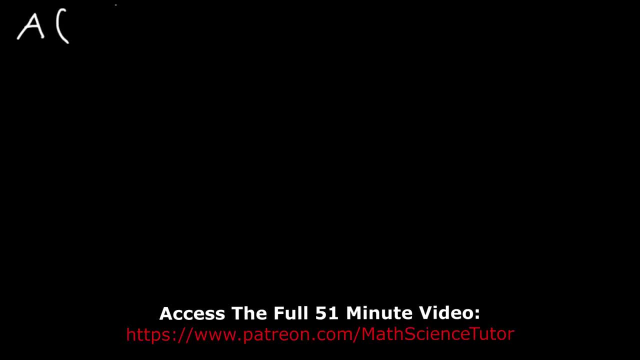 question for you. let's say, if we have the initial point a, which is that negative 1, negative 3, and you're given the vector V, which is the directed line segment from a to b, and let's say it's 3i minus 2j, 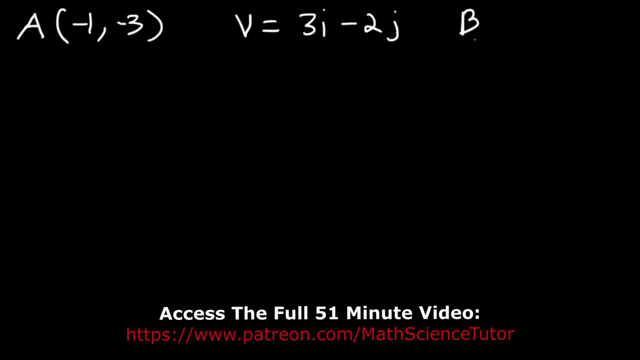 what is point b? if a is the initial point and b is a terminal point, how can you use vector V to find the answer? well, you can get the answer graphically. first let's plot a vector a so it's at negative 1, negative 3, and then we can use vector V to find point B. so notice. 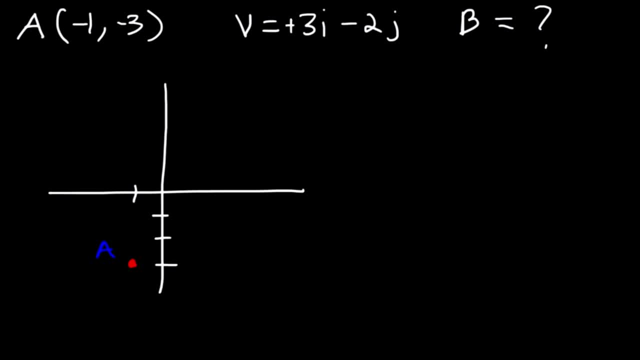 that we have positive 3i. That means from A we need to travel 3 units to the right, So we're at an x value of negative 1.. If we add 3 to it, it's going to take us to this point here. So we travel 3 units to the right. 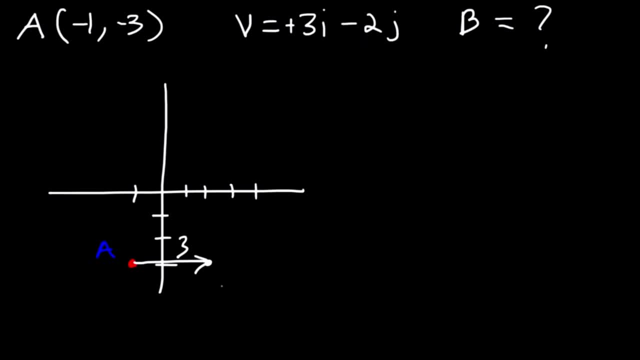 Now notice that there's a negative 2 in front of J, which means we need to go down 2 units. So therefore, this is point B. Point B is located at an x value of 2 and a y value of negative 5.. 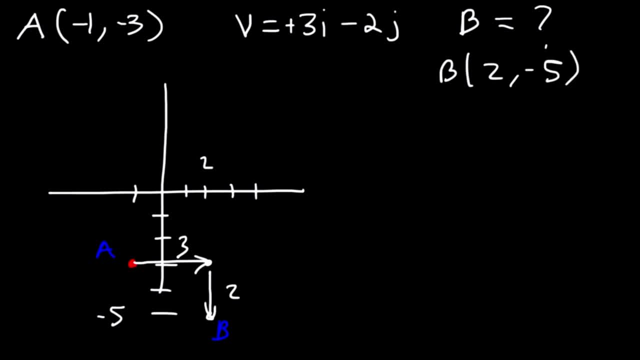 So, basically, if you have the initial point A and you want to find the terminal point B, all you've got to do is simply add 3i or 3 to negative 1, and also add negative 2 to the y value, negative 3.. And then you'll get the 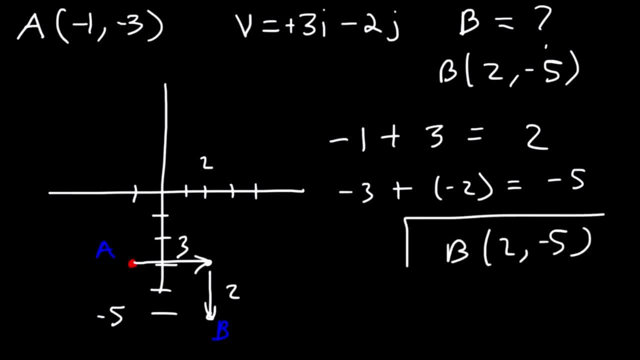 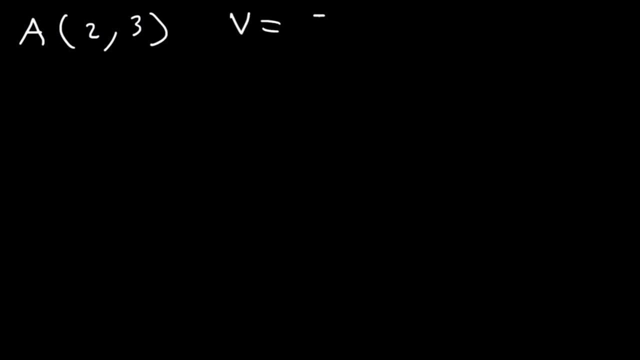 point 2.. So that's how you can find the terminal point from the initial point. Let's try another example like that. So let's say the initial point A is 2, 3. And vector V? let's say it's. 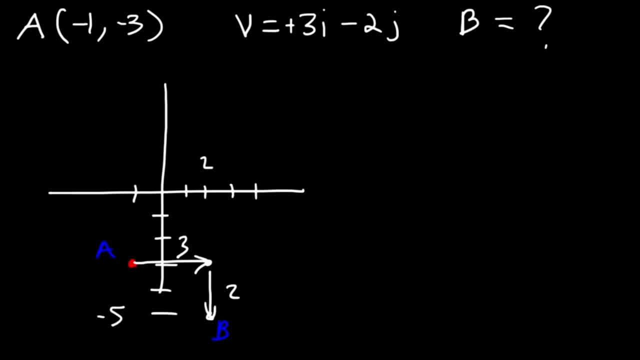 Point B is located at an x value of 2 and a y value of negative 5.. So, basically, if you have the initial point A and you want to find the terminal point B, all you got to do is simply add 3i or 3 to negative 1, and also add negative 2,. 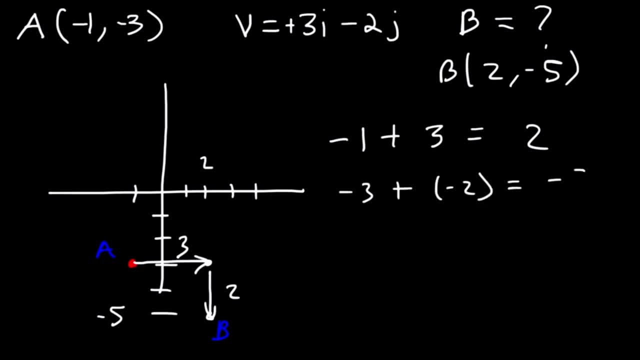 to the y value negative 3.. And then you'll get the point 2, negative 5.. So that's how you can find the terminal point from the initial point. Let's try another example like that. So let's say the initial point A is 2, 3.. 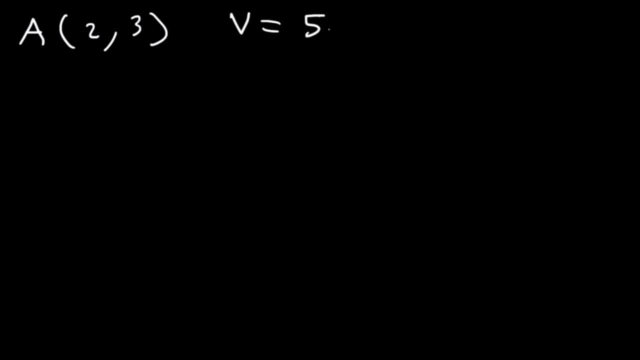 And vector V. let's say it's 5i minus 4j. Find the terminal point B. So a quick and simple way is you could use a form if you want. Vector V is x2 minus x1, and it's also y2 minus y1 times j. 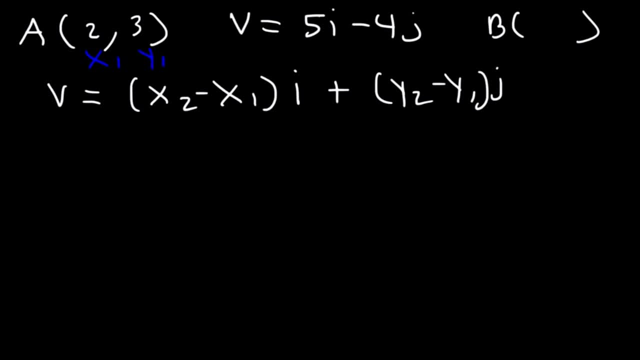 So keep this in mind. This is x1, y1.. That's the initial point. We need to find x2 and y2.. So vector V is 5i minus 4j, And that's equal to x2 minus x1, and x1 is 2.. 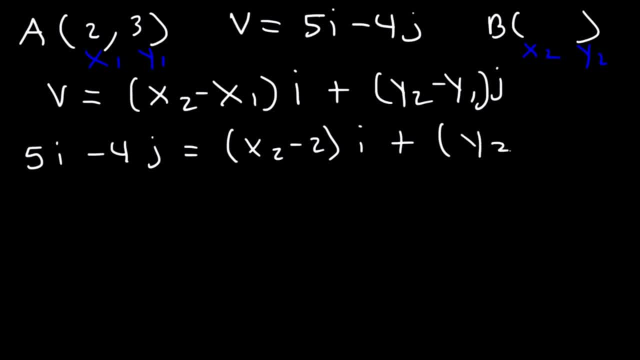 And y2 minus y1.. We're looking for y2, y1 is 3.. So what we need to do is set 5 equal to x2 minus 2, because they're associated with the same variable i, or the same letter i. 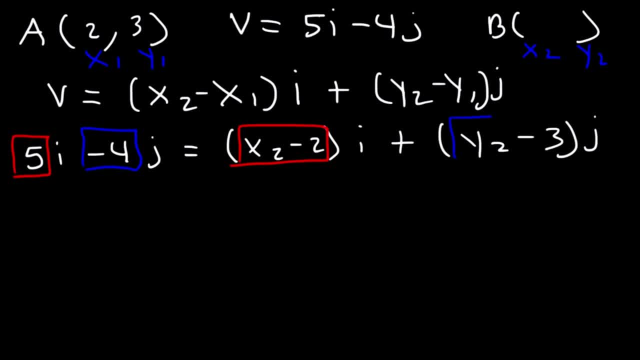 And we have to set negative 4 equal to y2 minus x2.. So we're going to add 3 to get x2.. So 5 is equal to x2 minus 2.. So basically we have to add 2 to 5 to get x2, the terminal point. 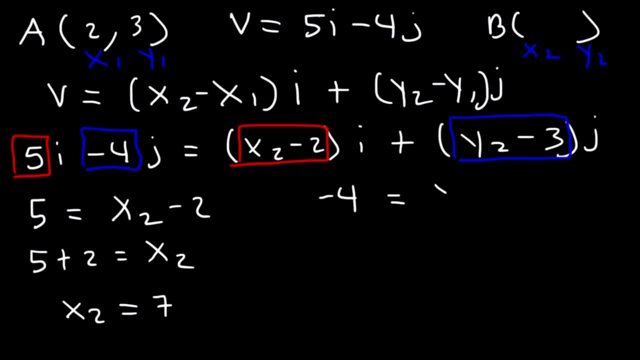 So x2 is 7.. Next let's set negative 4 equal to y2 minus 3.. If we add 3, negative 4 plus 3, that will give us a y2 value of negative 1. So therefore, point B is 7,. 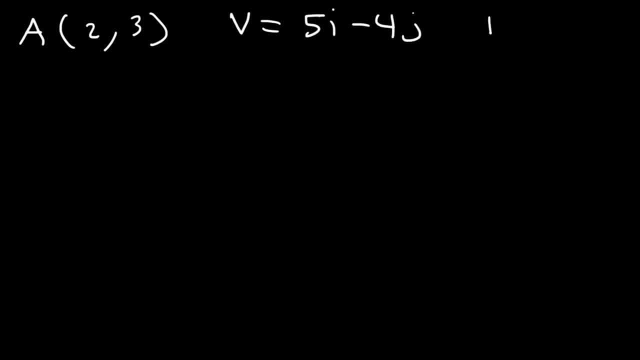 5i minus 4j. Find the terminal point B. So a quick and simple way is you could use a formula if you want. Vector V is x2 minus 3.. minus x1.. And it's also y2 minus y1 times j. 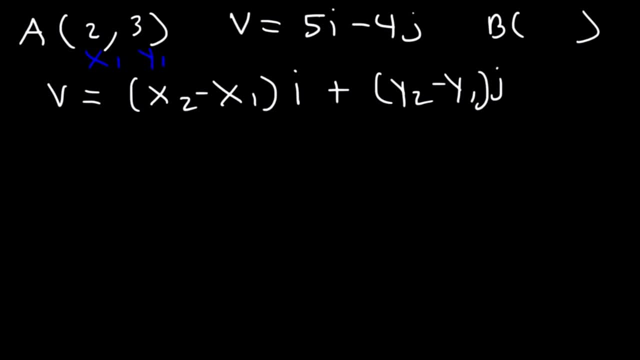 So keep this in mind. This is x1, y1.. That's the initial point. We need to find x2 and y2.. So vector V is 5i minus 4j, And that's equal to x2 minus x1.. 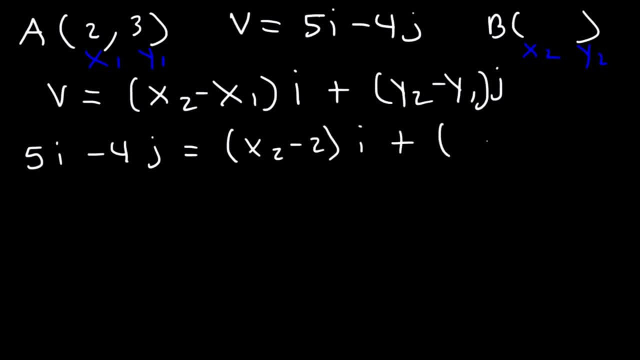 And x1 is 2. And y2 minus y1.. We're looking for y2.. y1 is 3.. So what we need to do is set 5 equal to x2 minus 2.. Because they're associated with the same variable. 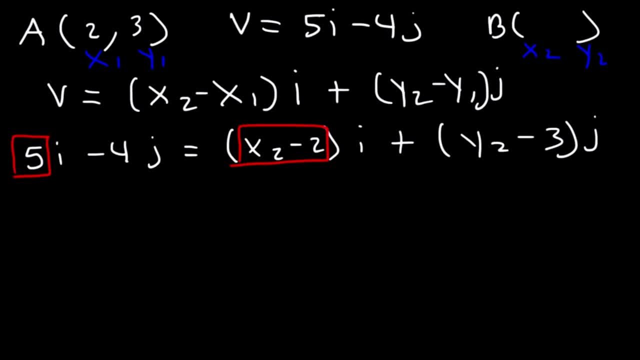 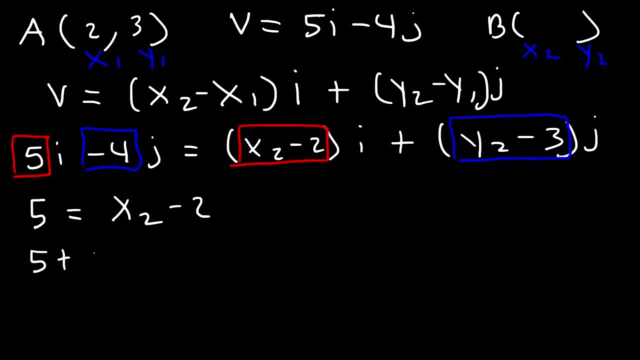 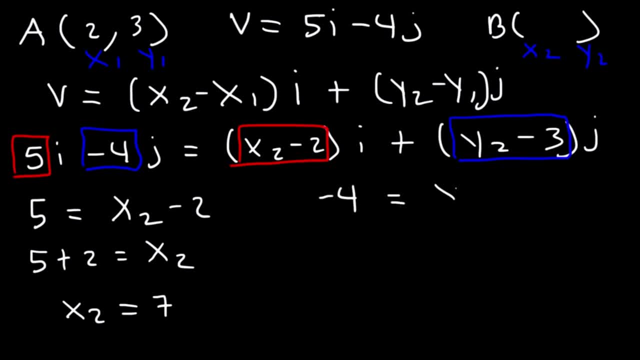 So x2 is 7.. Next let's set negative 4 equal to y2 minus 3.. If we add 3, negative 4 plus 3, that will give us a y2 value of negative 1.. So therefore point B is 7 comma, negative 1.. So if you add 2 plus 5, you get 7.. So if you add 2 plus 5, you get 7.. So if you add 2 plus 5, you get 7.. And 3 plus negative 4, you get negative 1.. 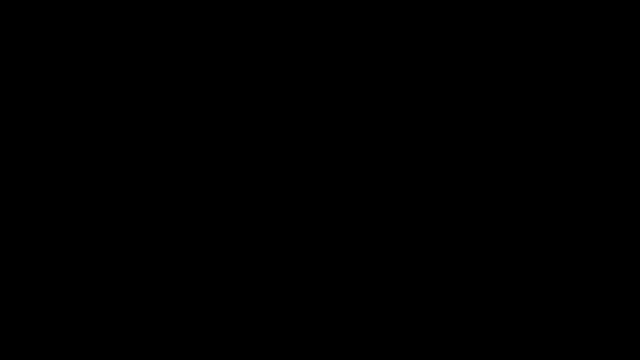 And 3 plus negative 4, you get negative 1.. Now let's say, if we're looking for the initial point A, And let's say the vector v is negative, 3i plus 4j And the terminal point is: 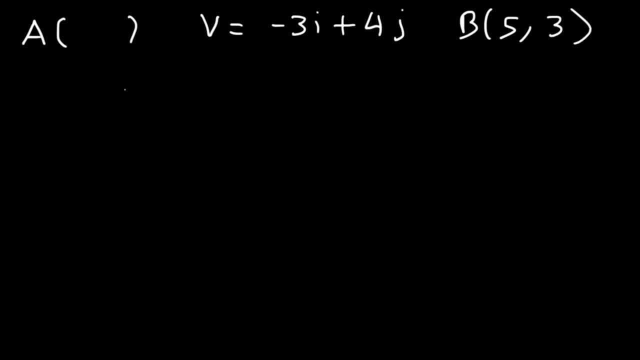 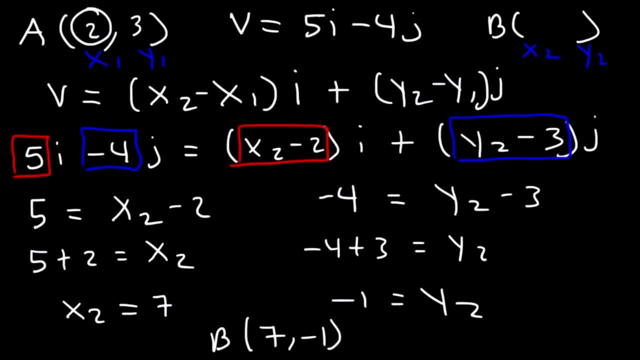 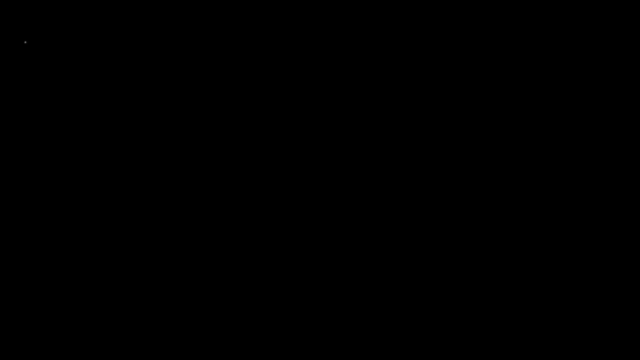 comma negative 1.. So if you add 2 plus 5, you get 7.. And 3 plus negative 4, you get negative 1.. Now let's say, if we're looking for the initial point A And let's say the vector V is negative, 3i plus 4j. 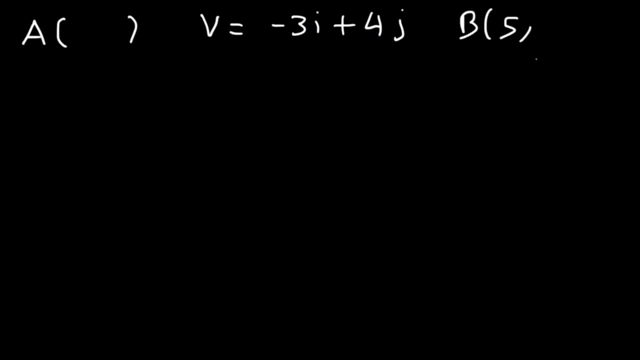 And the terminal point is 5, 3.. Find the initial point A. So keep in mind you can use the formula. The vector V is equal to x2 minus x1i plus y2 minus y1j, And it's always good to define where everything is. 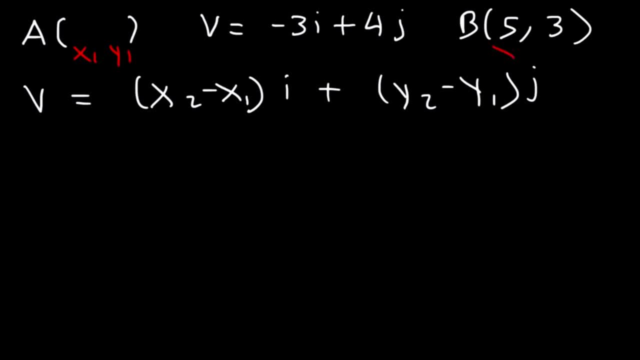 So this is x1 and y1.. That's what we're looking for in this problem, And the terminal point B is x2y2.. So the vector V is negative 3i plus 4j, And that's equal to x2, which is 5.. 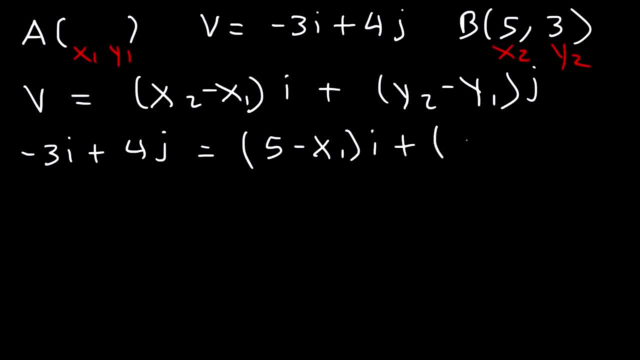 Minus x1 times i, Plus y2, which is 3.. Minus y1 times j, So this time we're going to set negative 3 equal to 5 minus x1.. That's associated with the i values. 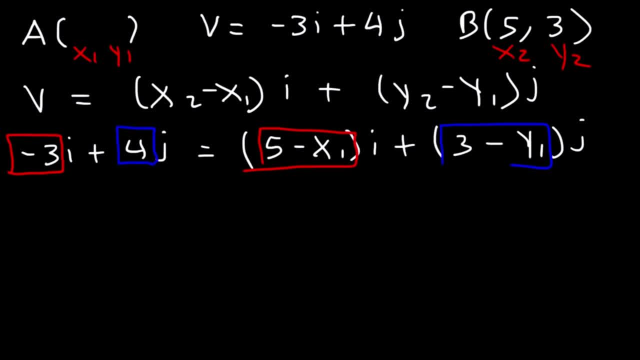 And for the j values, we're going to set 4 equal to 3 minus y1.. And let's find x1.. So what I'm going to do is subtract both sides By 5.. So negative 8 is equal to negative x1.. 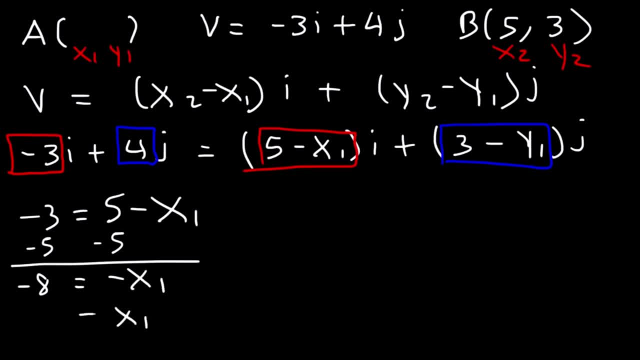 And then, if we multiply both sides by negative 1, x1 is equal to positive 8.. Now let's set 4 equal to 3 minus y1.. And let's subtract both sides by 3.. 4 minus 3 is 1.. 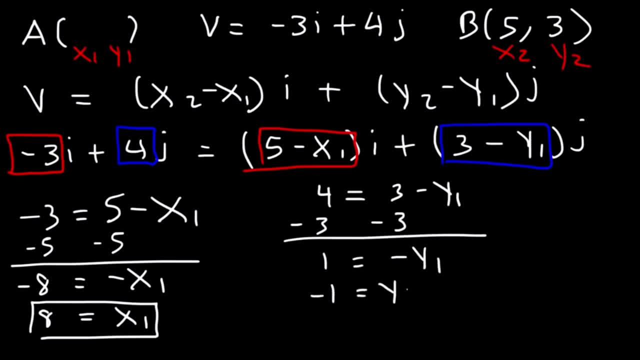 And if we multiply both sides by negative 1, negative 1 is equal to y1.. So therefore the initial point A is 8 comma, negative 1.. Now let's say, if you're given an initial point in three directions, 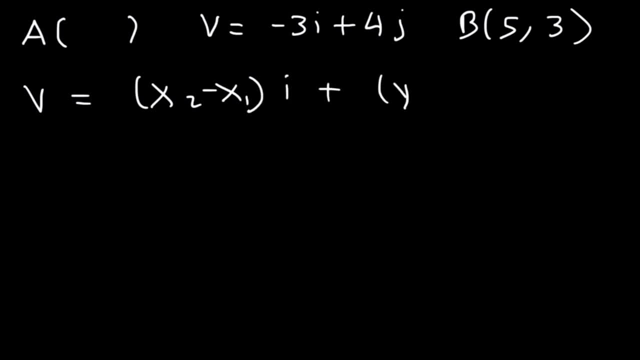 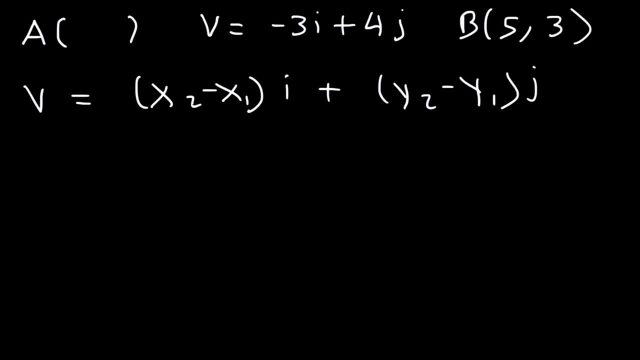 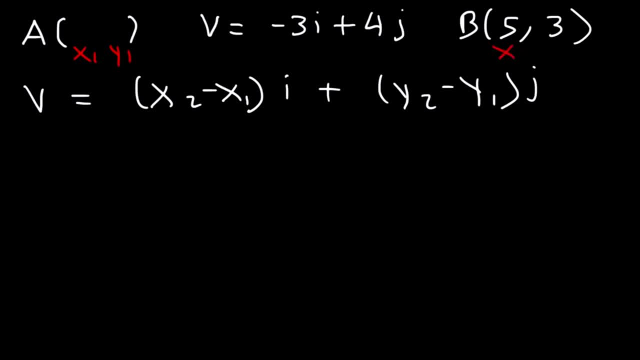 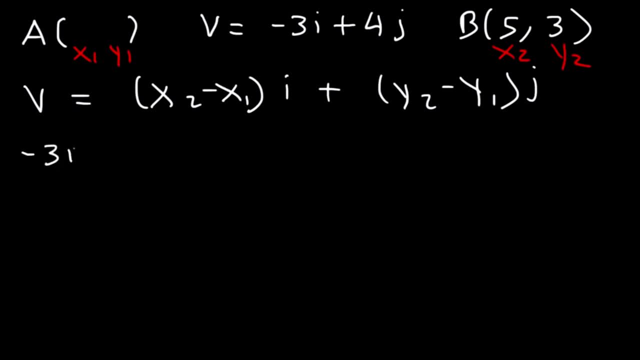 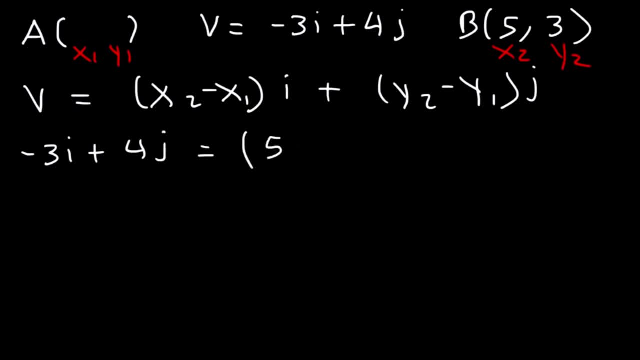 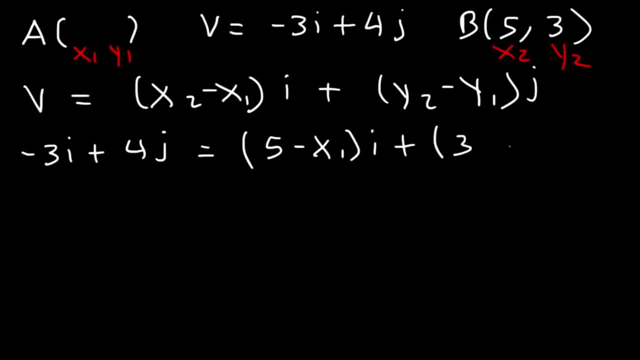 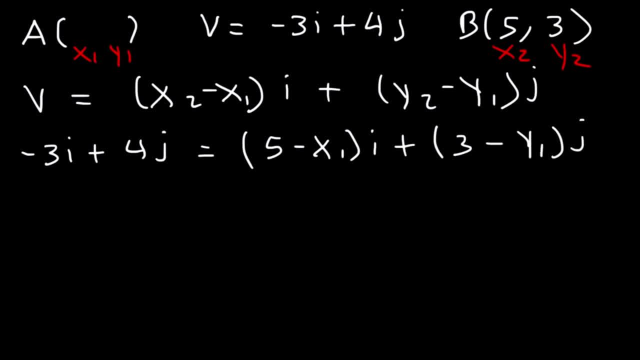 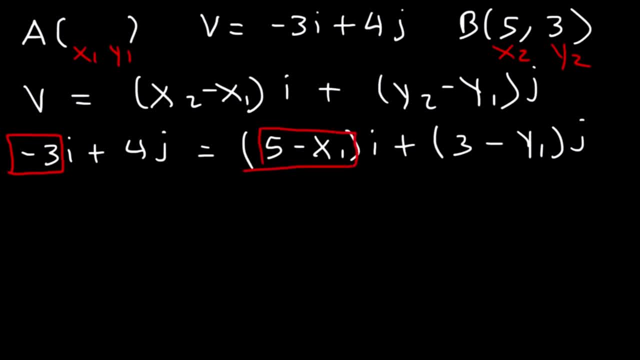 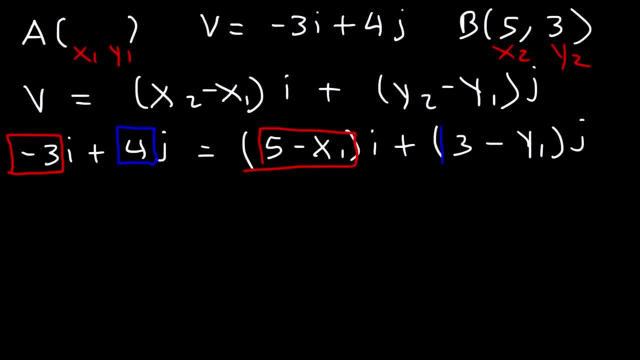 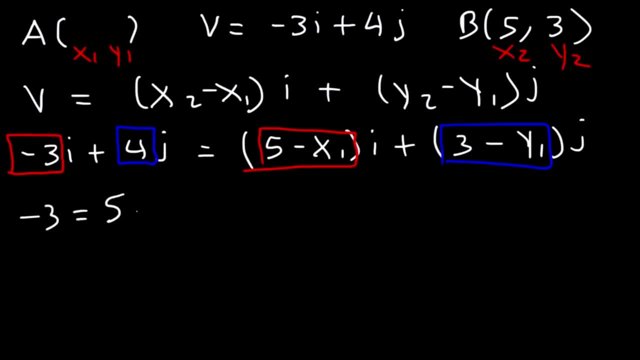 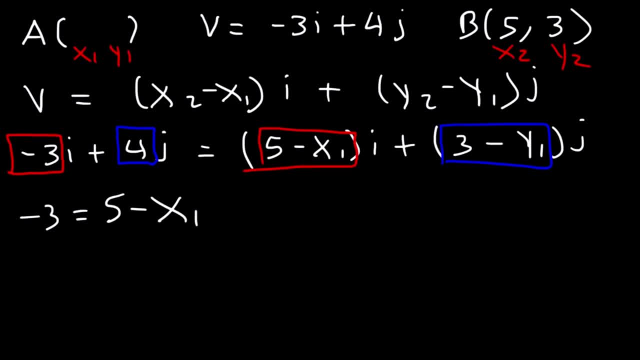 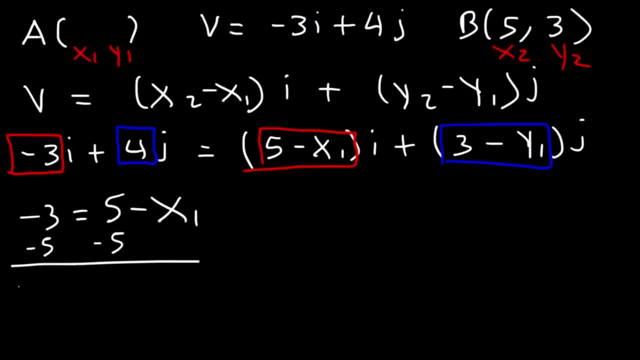 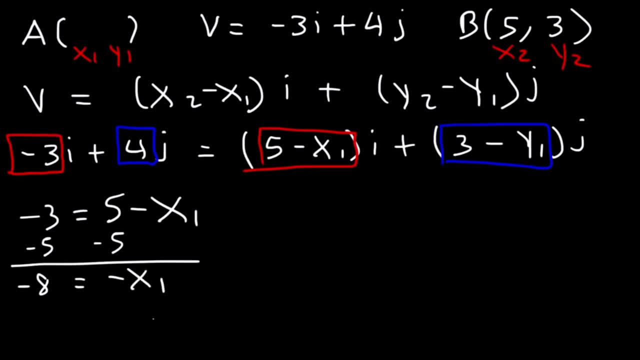 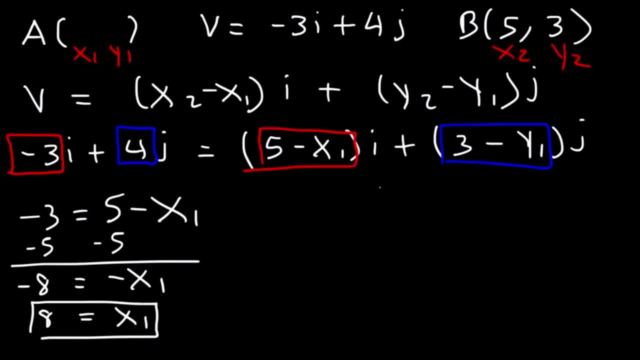 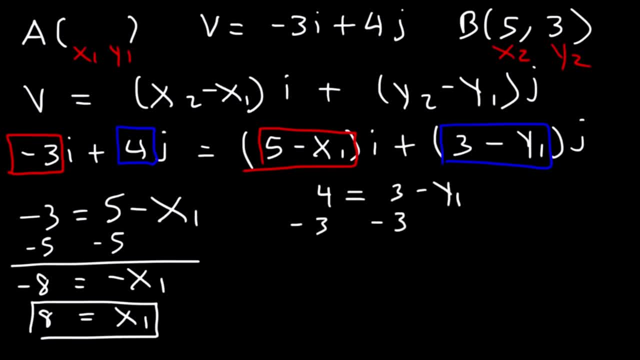 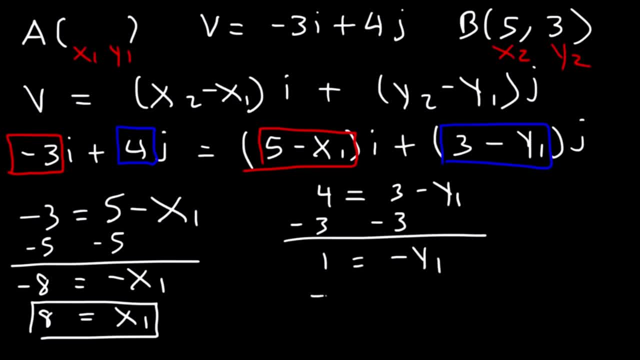 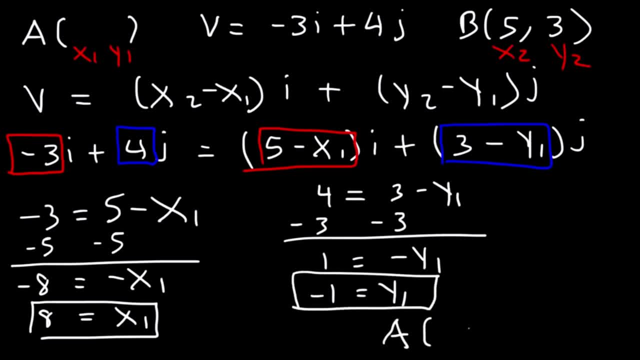 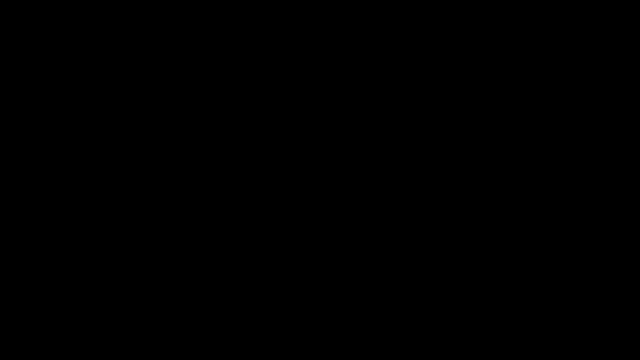 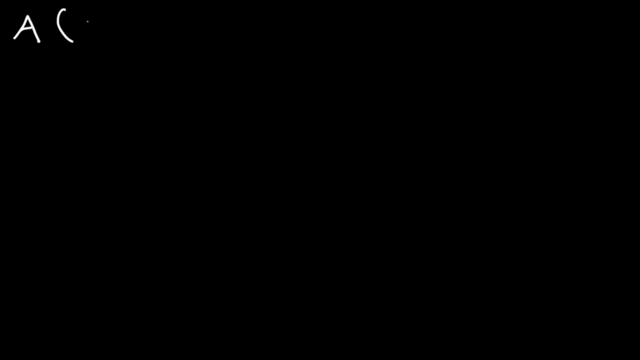 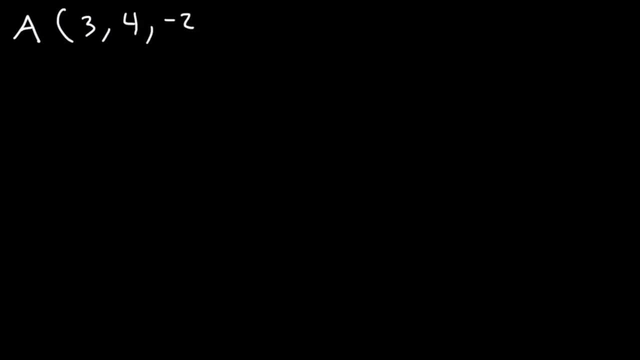 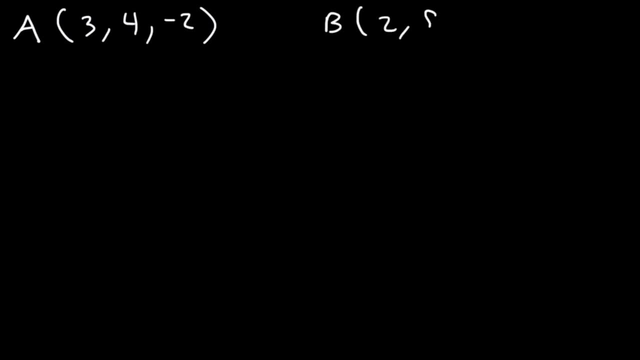 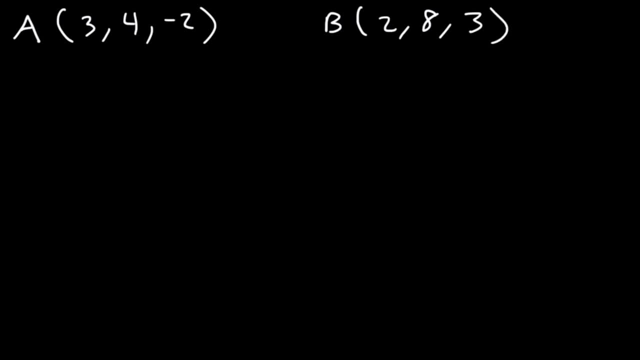 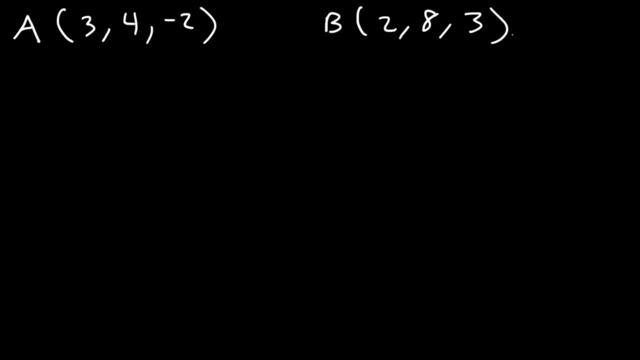 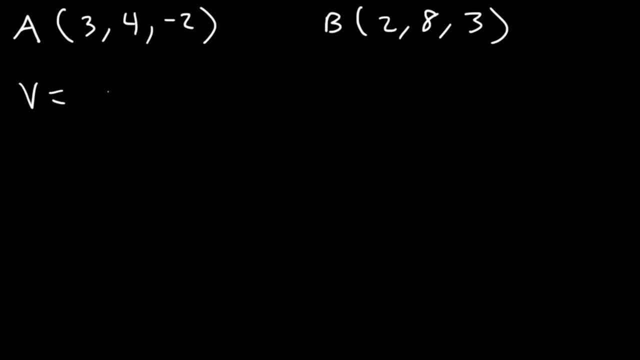 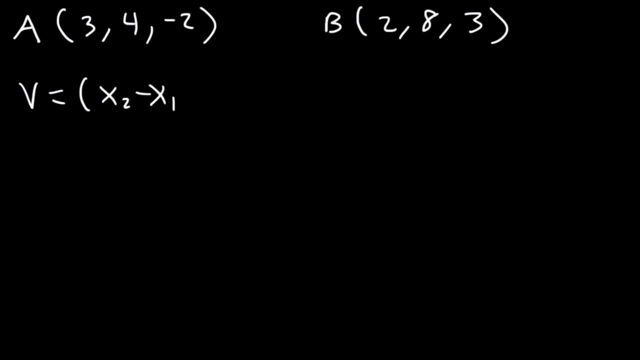 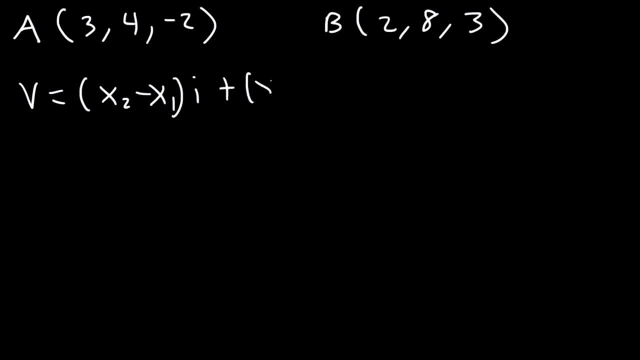 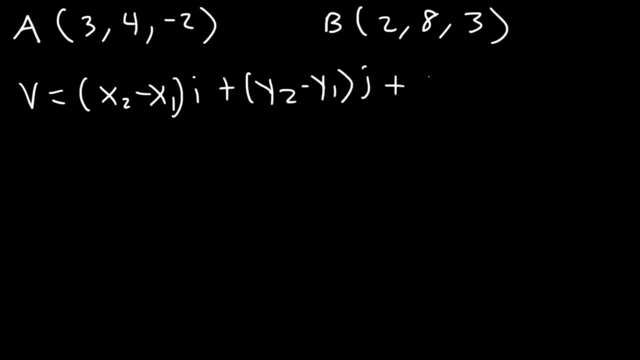 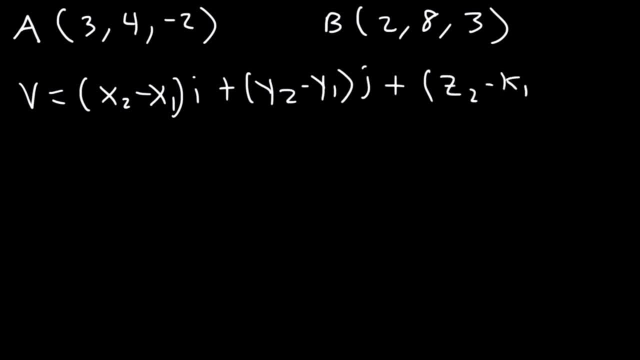 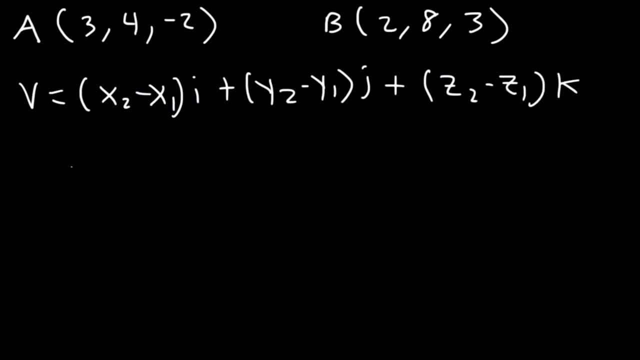 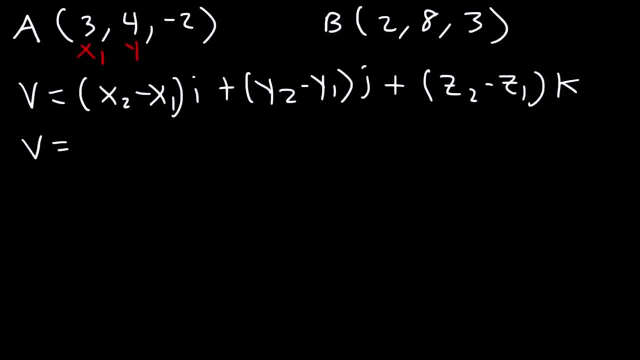 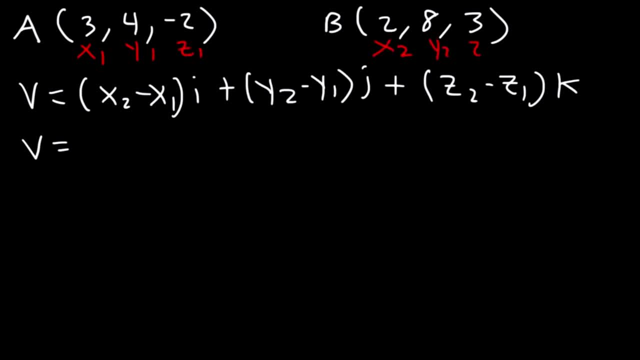 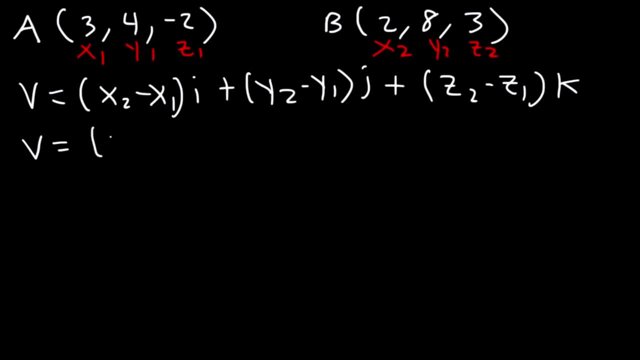 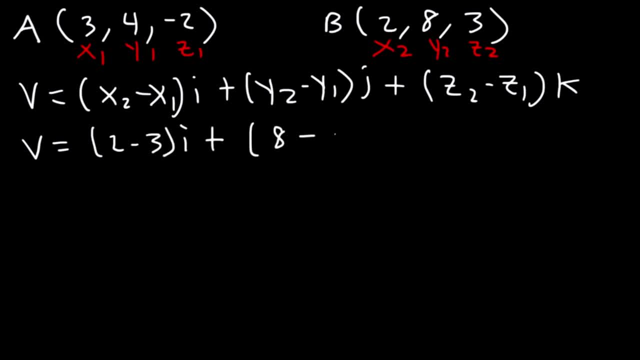 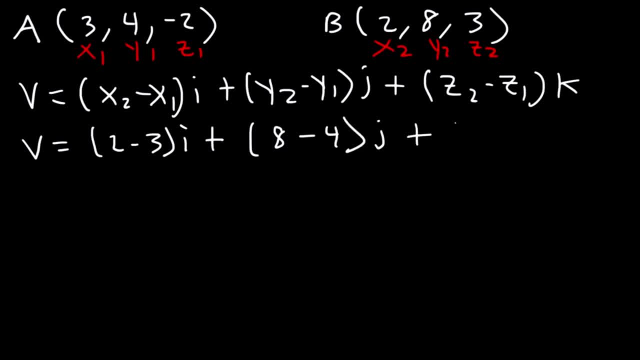 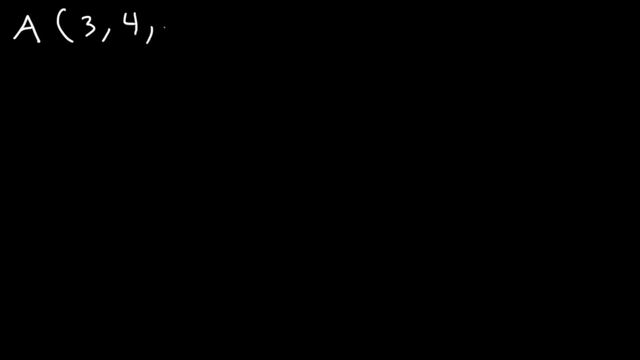 Let's say you have the x value, the y value and the z value And you're given the terminal point as well. Find the vector v and express it in component form, That is, in i, j and k. And also find the vector v in component form. 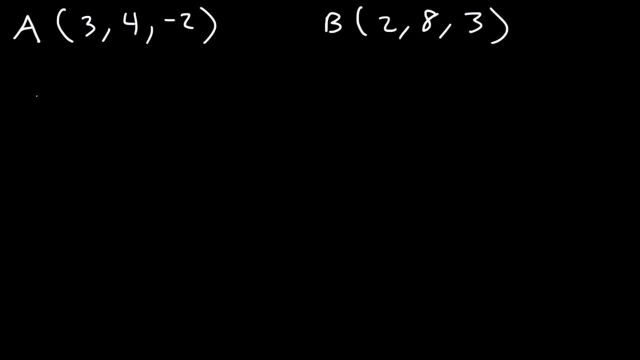 Find the vector v in component form And also find the magnitude of vector v. So vector v is going to be the difference in the x values That's going to give us the x component, And then the difference in the y values will give us the number in front of j. 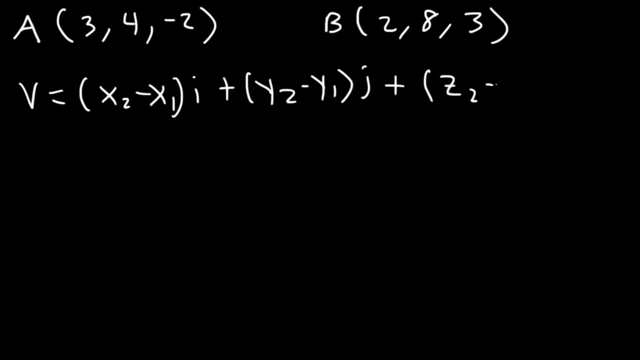 And the difference in the z values will give us the number in front of k. So this is x1, y1, z1.. And this is x2, y2, and z2.. So x2 minus x1, that's going to be 2 minus 3.. 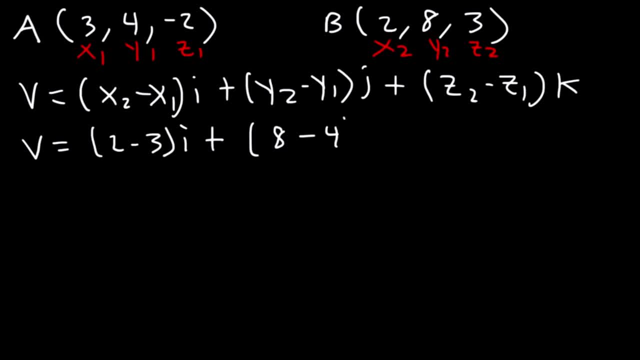 y2 minus y1, that's 8 minus 4.. And then we have z2 minus z1,, that's 3 minus negative 2. So 2 minus 3 is negative 2.. So 2 minus 3 is negative 1.. 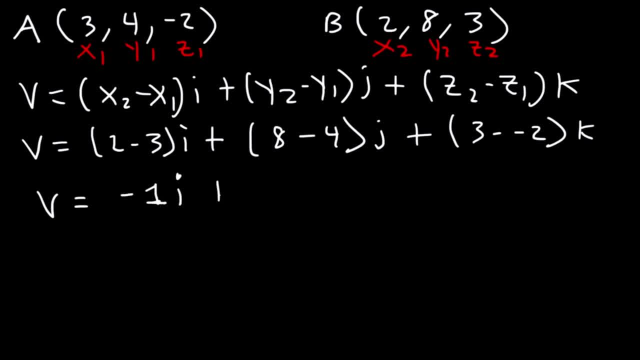 So we got negative 1 times i, And 8 minus 4 is 4.. 3 minus negative 2 is 5.. So the vector v is negative 1i plus 4j plus 5k, Which we can represent as negative 1 comma, 4 comma, 5.. 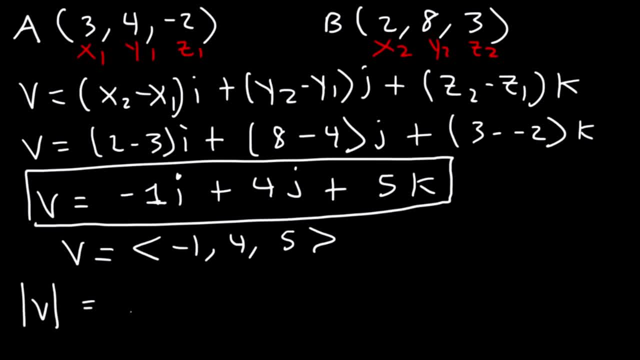 Now to find the magnitude, it's simply the x component squared plus the square of the y component squared Plus the square of the z component, all within the square root. So it's going to be the square of negative 1 plus the square of 4 plus the square of 5.. 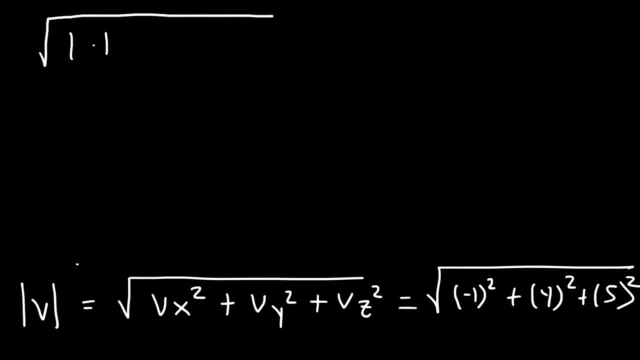 Negative: 1 squared is just 1.. 4 squared is 16.. 5 squared is 25.. 1 plus 16.. 16 is 17. And 17 plus 25, that's 42. And we can't simplify the square root of 42.. 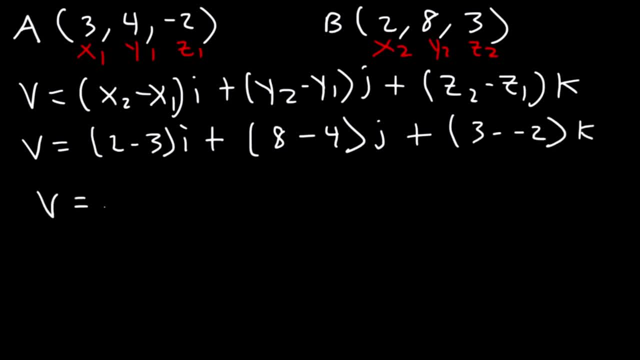 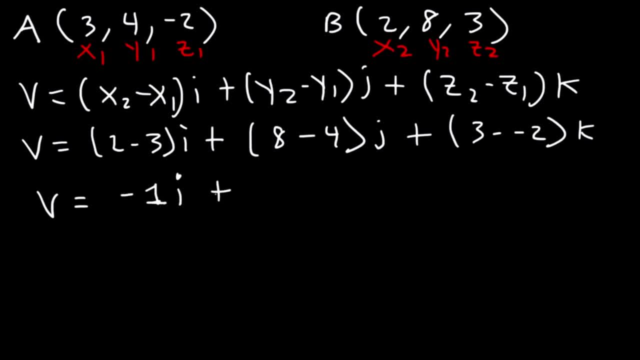 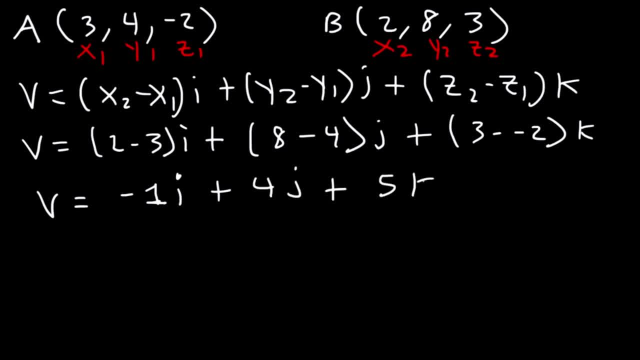 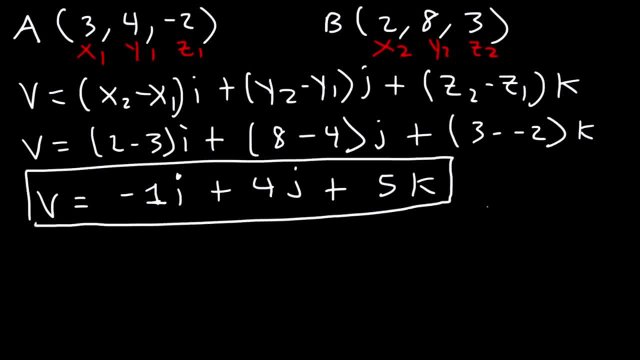 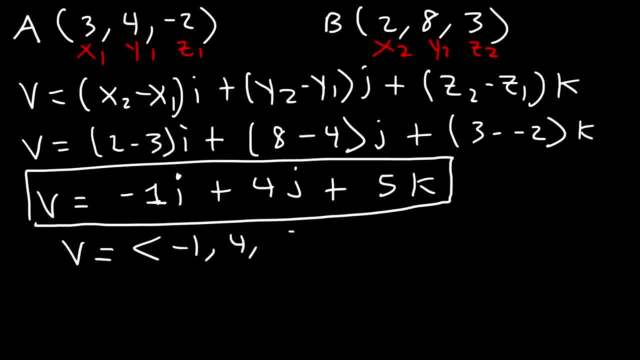 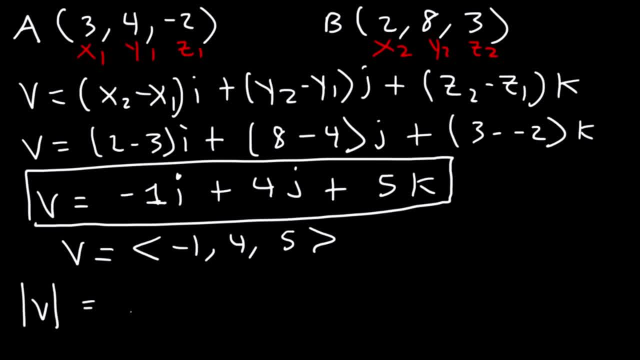 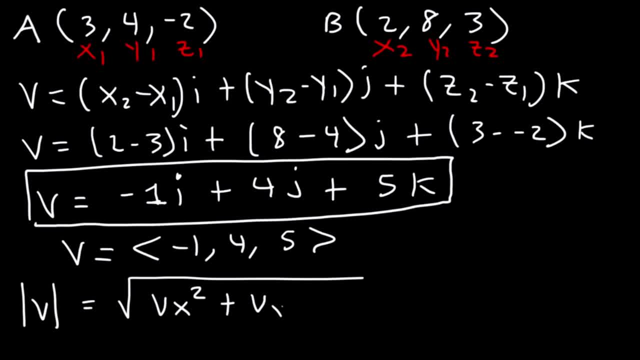 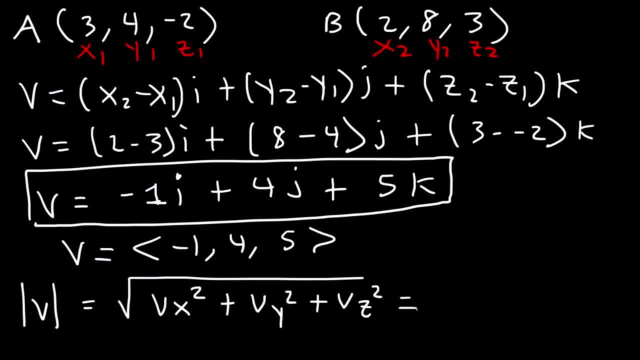 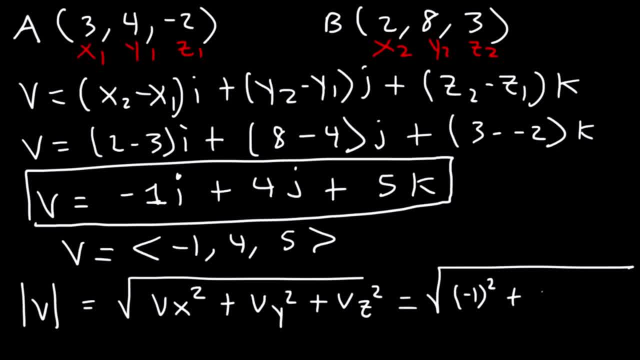 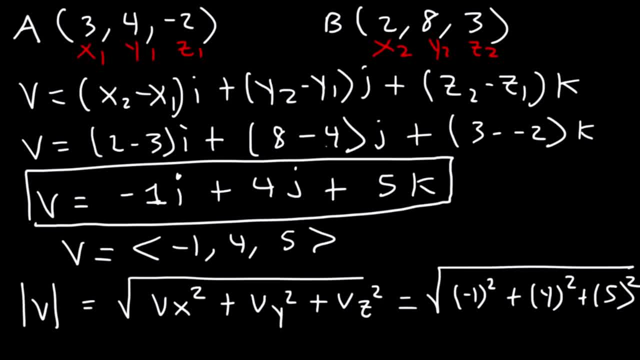 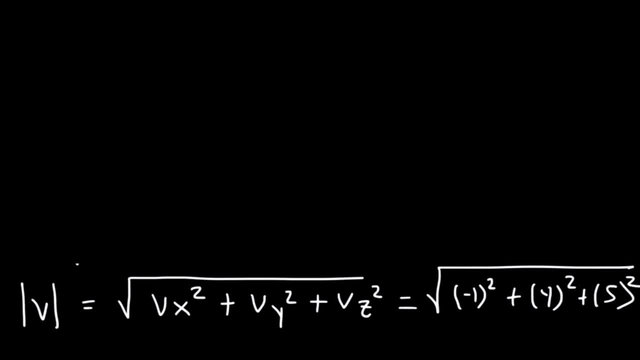 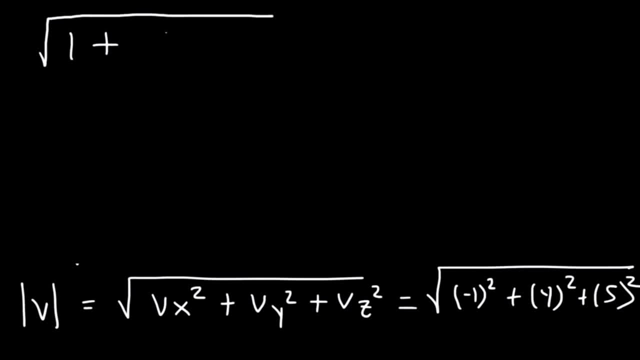 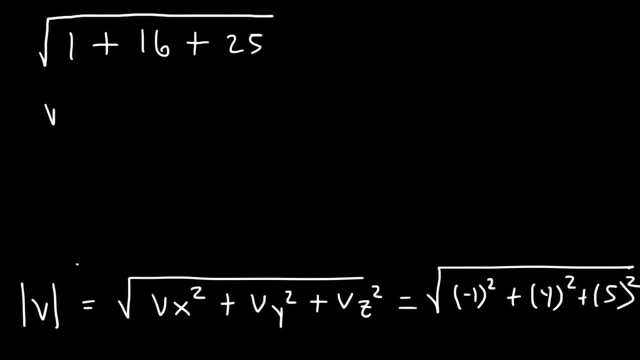 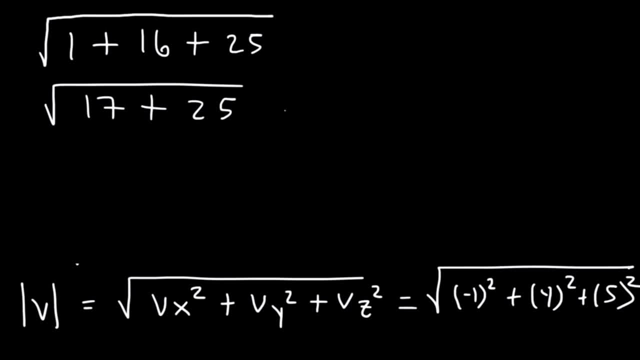 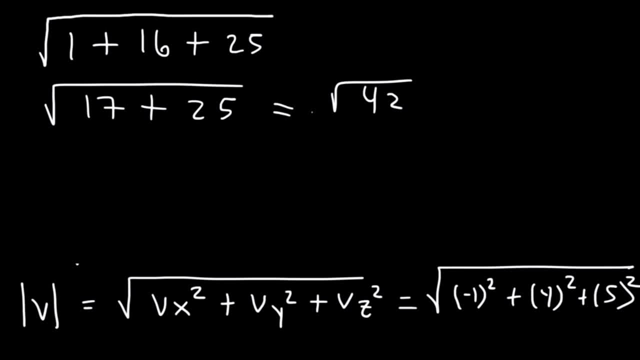 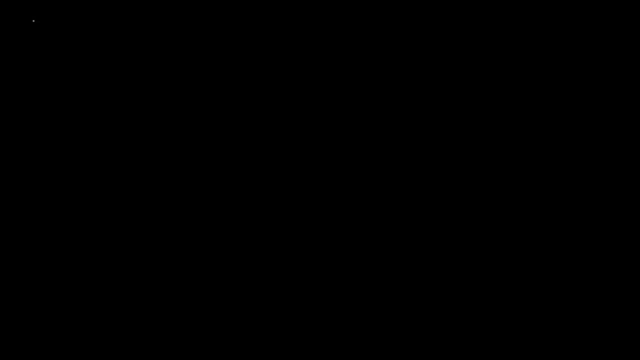 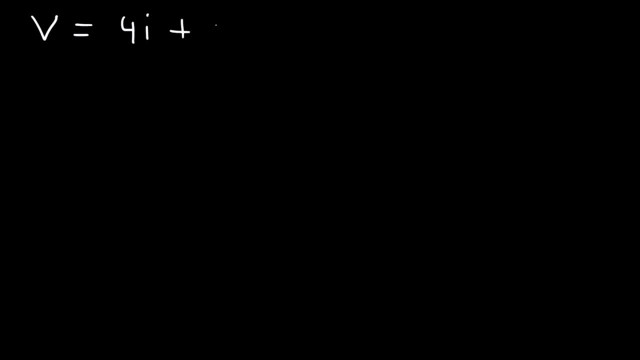 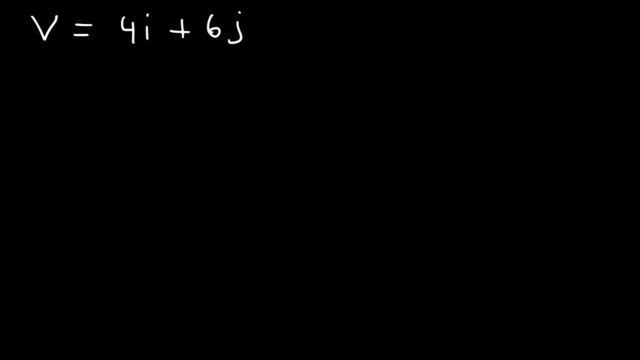 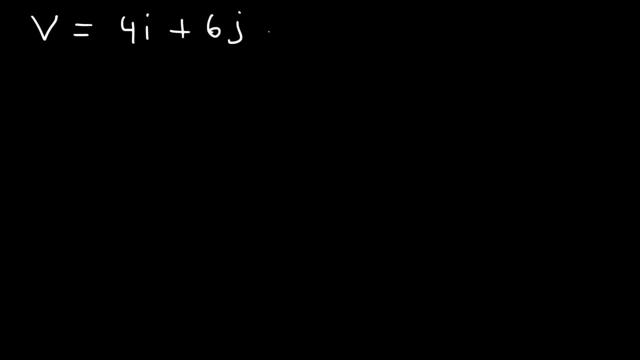 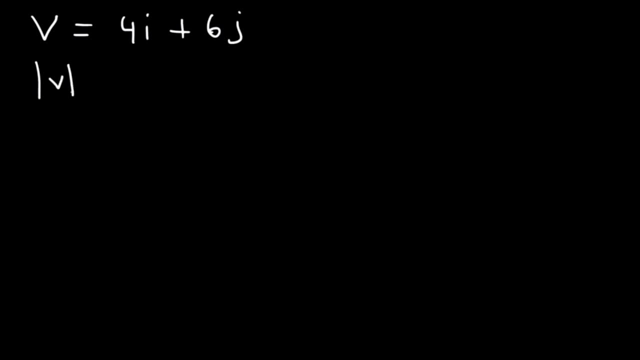 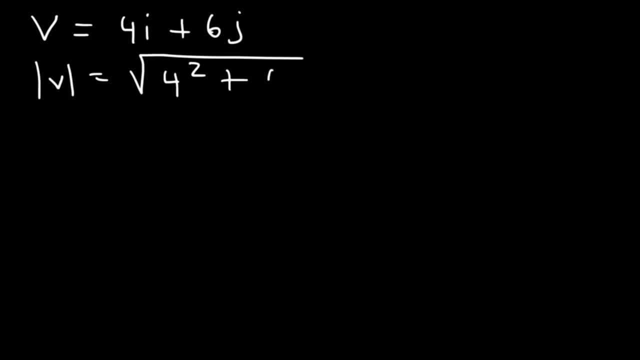 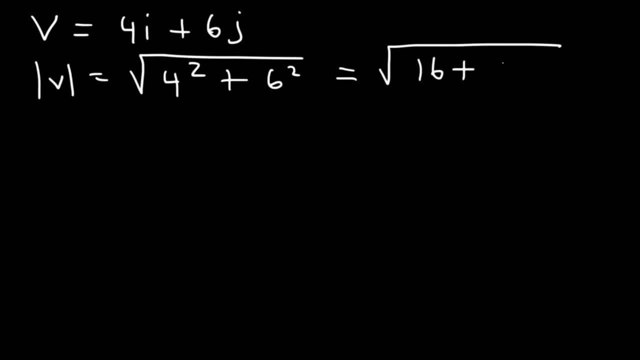 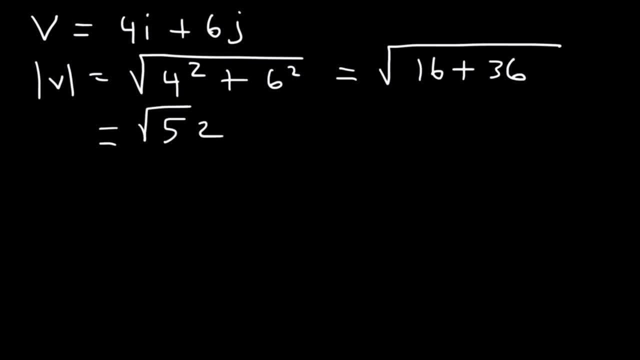 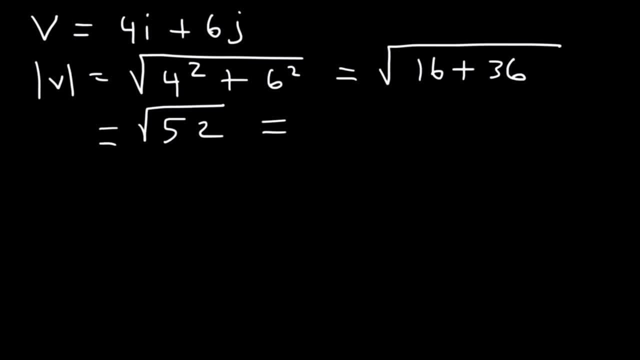 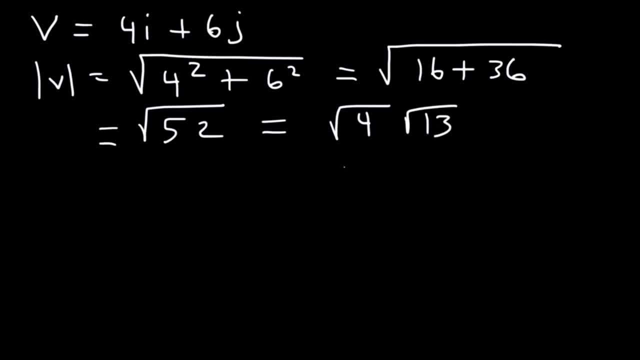 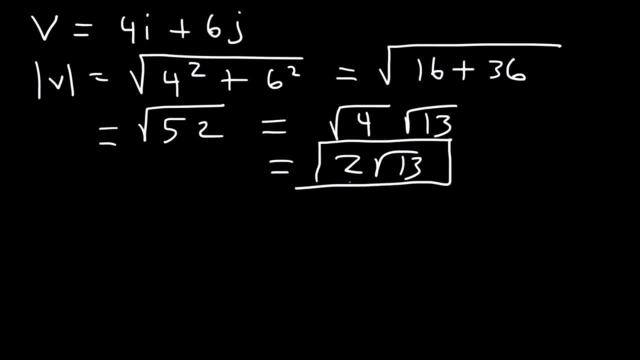 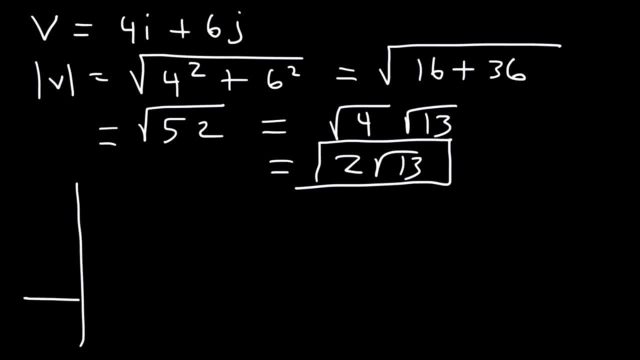 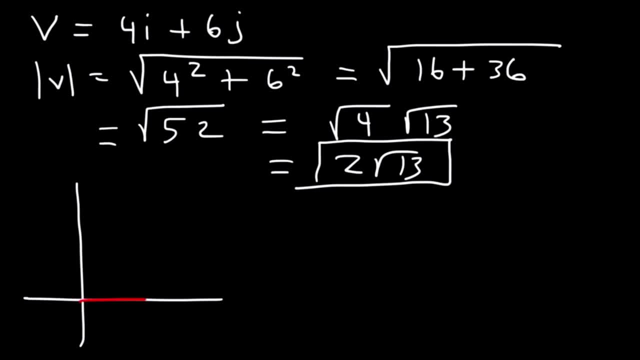 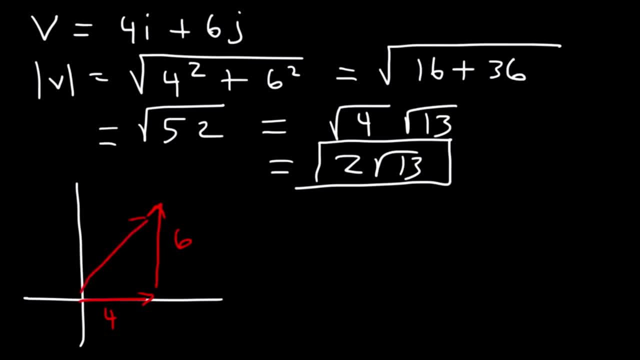 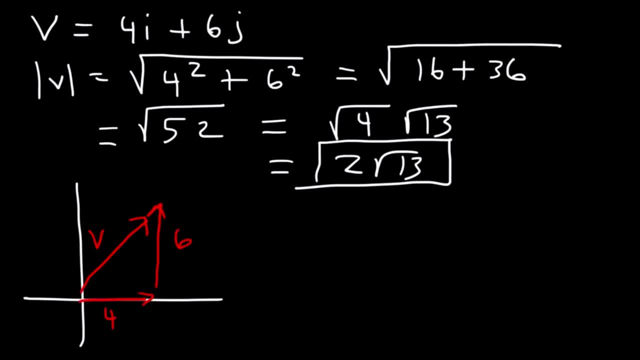 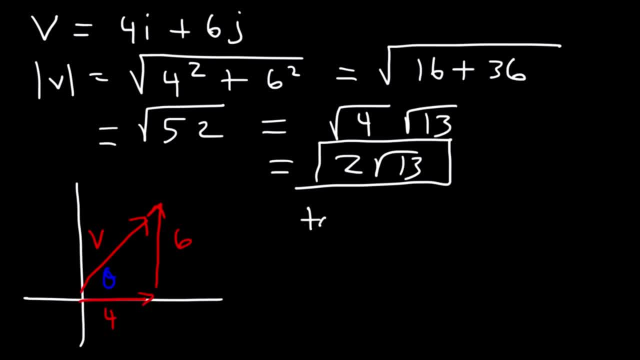 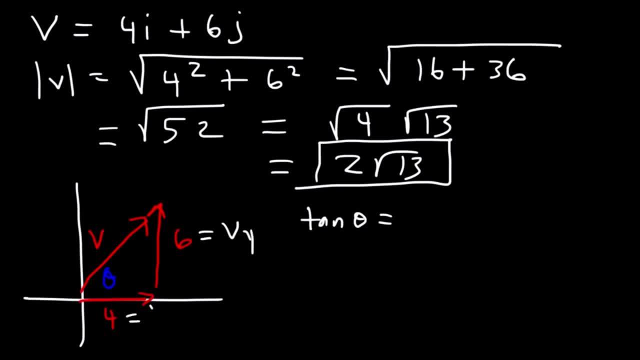 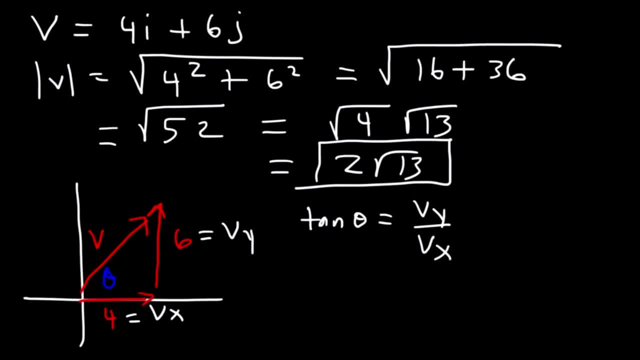 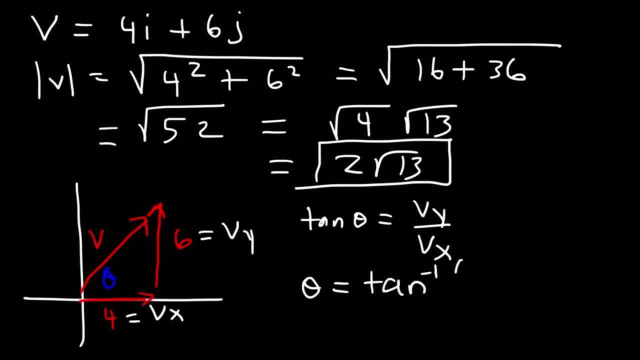